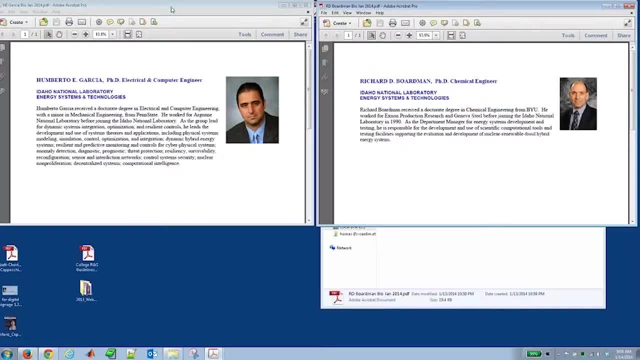 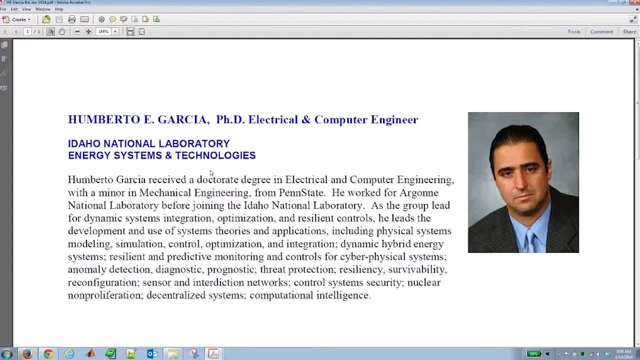 What I'll do now is go ahead and introduce our speakers. First of all, I'll go ahead and introduce Humberto, and he has a doctorate degree in electrical and computer engineering with a minor in mechanical engineering. Humberto, I don't understand How can you get a minor in mechanical engineering and still do electrical engineering? It sounds like you were a glutton for punishment there. 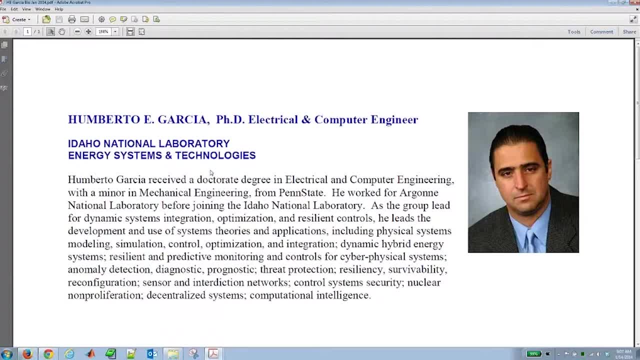 Actually, I got the funding from the nuclear engineering department, so I was engaged right from the beginning in a very multidisciplinary education. Oh, fantastic, Okay, well, so we are having a little bit of feedback now. Let me just mute some microphones here as we go. 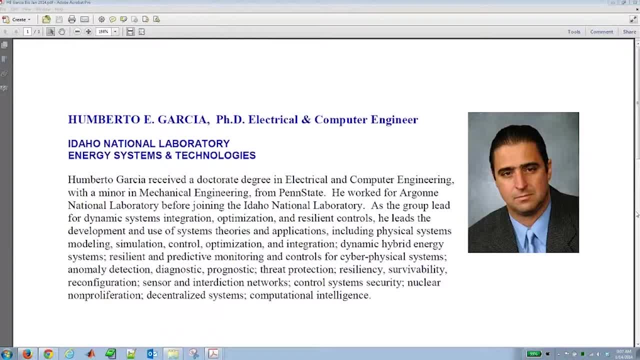 Okay. Okay, so if I've muted your microphone, feel free to unmute your microphone. just by selecting the button over to the right, the red button, You can unmute it. So let me go ahead and just continue with Humberto's introduction. Humberto has worked for Argonne and also INL and he's also right now the group lead for the dynamic systems integration, optimization, resilient control. 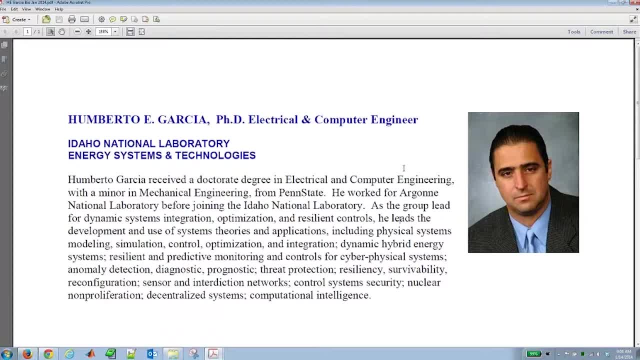 And you know, I've just got to say I went to a conference. Okay, I went to a conference there at Idaho National Labs or near there, and I'm very impressed by Humberto and his group and the things that he's working on. 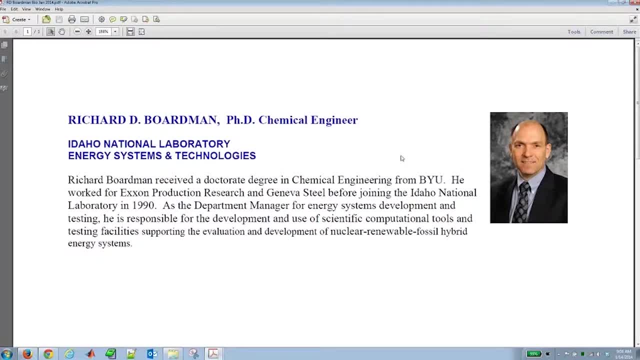 Okay, so let me switch over to Richard. Richard is on as well, and you know he has a doctorate degree from BYU in chemical engineering, and he worked for Exxon. I worked for Exxon too, Richard, so we have something in common there. 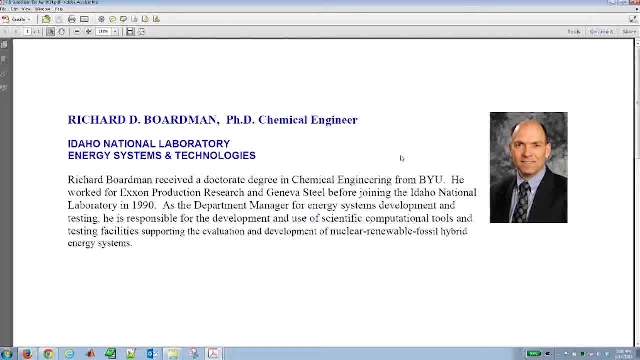 And then joined Idaho National Labs in 1990.. You know, the thing I'll say about Richard is he thinks big and the projects that he proposes and the things that he works on have a big impact, And you know. so I'm pleased to have Richard Humberto here. 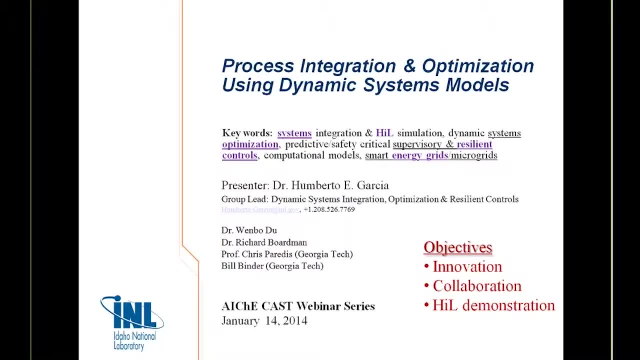 Well, let me just start this webinar by first thanking the American Institute of Chemical Engineers and, in particular, John, for the opportunity to brief you all, you guys, in some of the activities that we're doing. Thank you, Thank you. 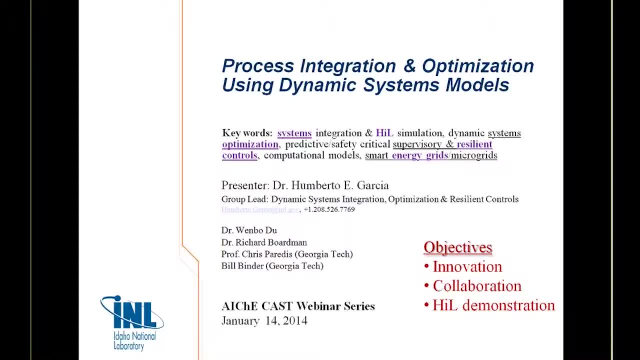 Thank you very much, abused by some of the activities that we're doing here at ANL. You know Richard is a coauthor of these presentations and also we have here Dr Khwebo Du, who is primarily from Michigan and he's an optimization expert. 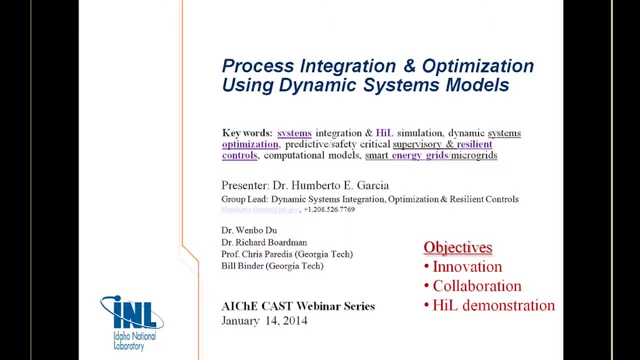 This effort also is in collaborations with Professor Chris Perez, Georgia Tech, and he's a student in Bill Binder. Thank you. A few things you will see in this presentation is key. notions are systems. We are interested in looking at the process and all technology solutions from a system. 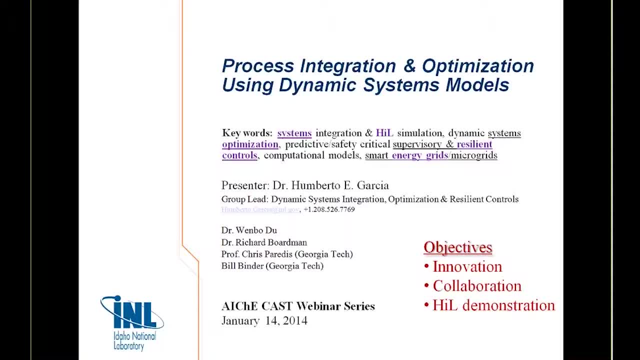 point of view, Also modeling, simulation, but also harrowing the loop. Another key word is optimizations and another one is controls. We are interested in, rather than power grids or smart power grids, more into energy grids in which you have a several community beside electricity. 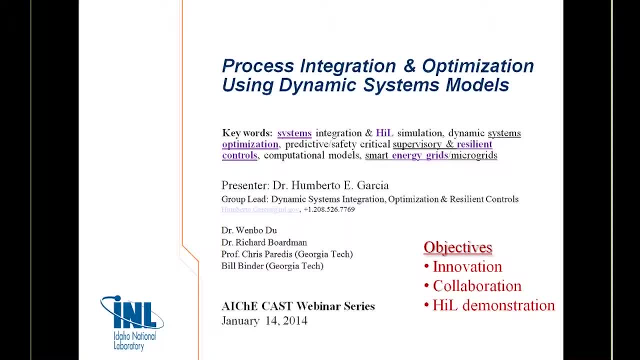 The key thing you will see here is the challenges as such that require innovation, not only in modeling and simulation, but also in control and optimization and integration of technology, Because the spectrum of the challenges are so wide. That's the kind of consortium we're trying to put together: not only national labs, but 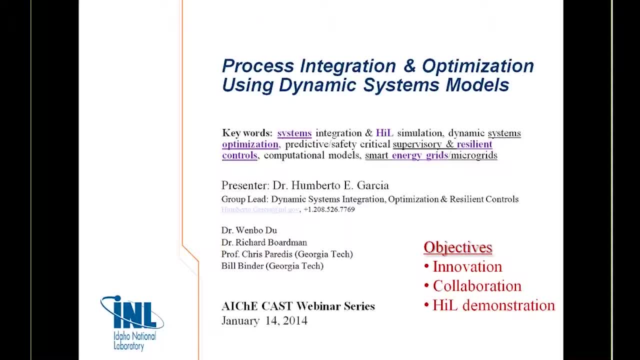 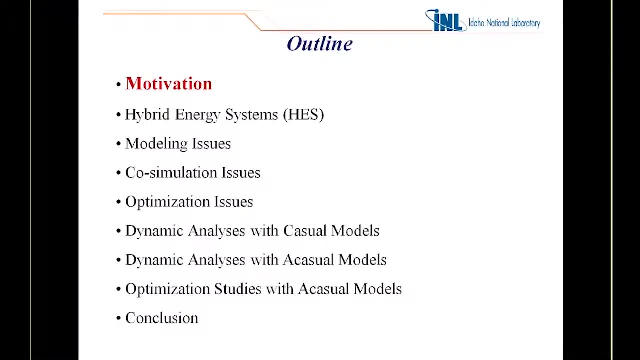 also university. Finally, it's harrowing the loop in demonstration because as we understand the system better and better, we want to be able to simulate the environment. The outline is a very brief motivation of what we're doing here, particularly in the energy systems. 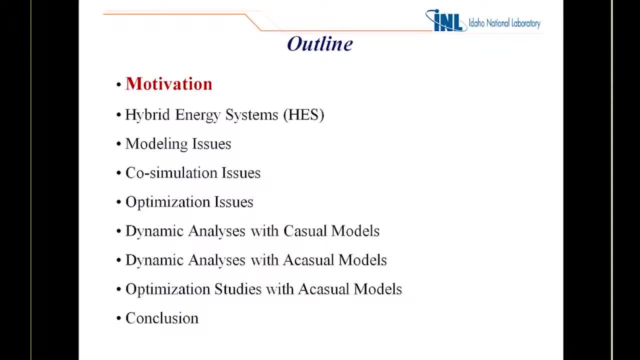 Then the concept of high-grade energy systems. Then some of the modeling issues, a challenge that we have facing and tackling. Then issues regarding simulation, in which you might have a number of models or physical assets all talking together coordinatedly. Then the issues regarding optimization, because at the end, we try to optimize the system, not 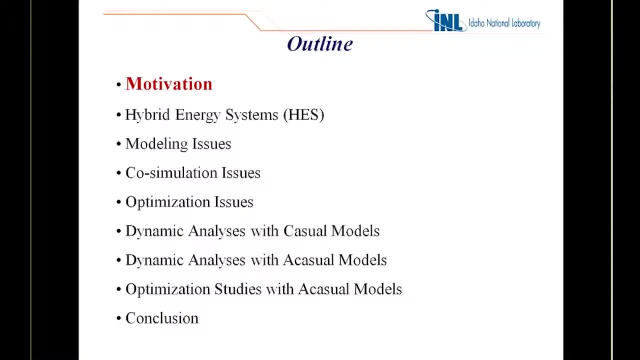 only in the design of the system- what kind of energy resources are needed- but also in how to operate the system. Then the last three ones give a few results. some of those results you can find it in publications out there. Then I conclude with the conclusions of future work. 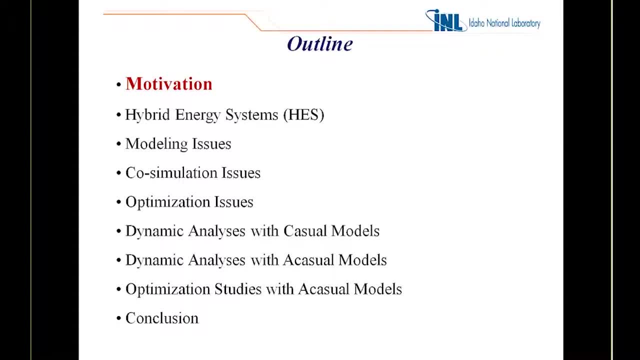 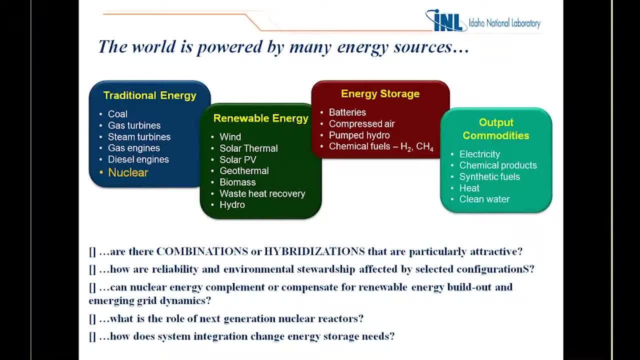 Please, as Joe indicated, interrupt me anytime you might have a question. The key part here is: well, we have all kinds of different energy resources, and not only source of energy, but also energy sources. I'm going to show you a few examples. 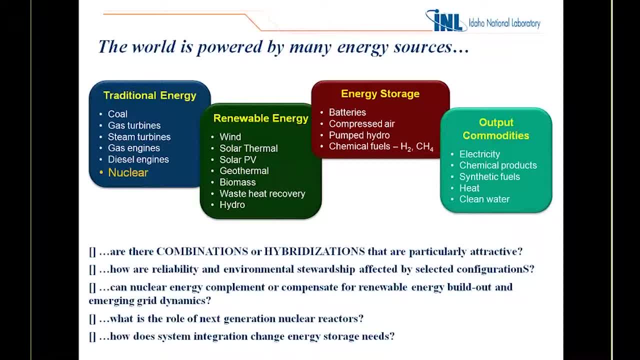 Here's a few examples. I'll give you a few examples. A couple of examples. We have the energy in both the solar and energy communities. Then we have the traditional energy- coal, gas, nuclear- Then we have these new elements. it's called renewable energy. 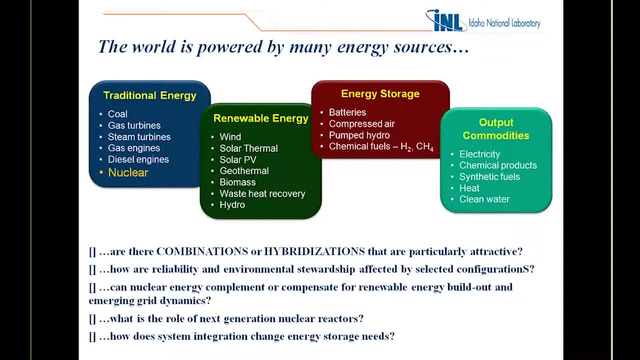 We have wind, hydro, we have solar, so forth, To deal with the availability of renewable, then there is need for some kind of energy storage. That might be electrical, or it could be thermal and many other ones. Then again, we utilize energy to create different sources. 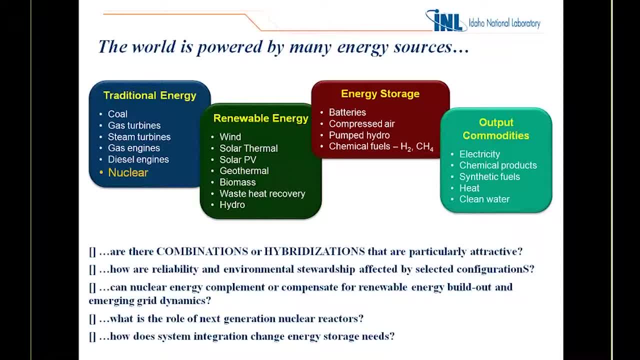 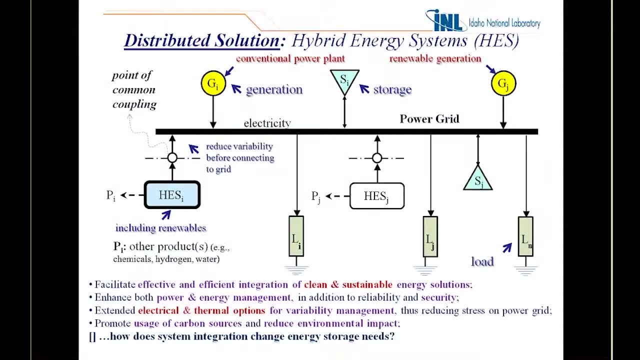 commodities. it could be electricity or could be synthetic fuel, and the question is: is what will be the optimal combination of these resources to meet certain requirements on this certain constraint- and again I'm going to go very fast for this introductory slide- then so if we look the the grid, so we 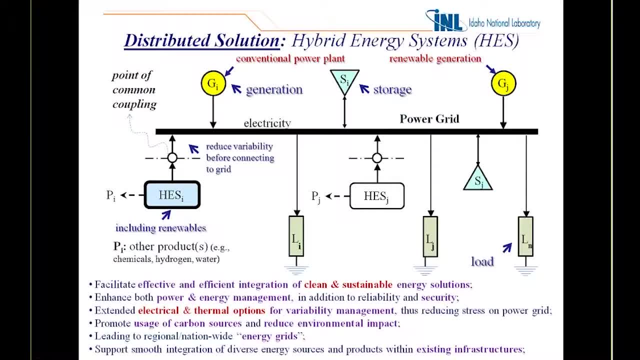 have all different resources interconnected by electrical grid and in traditional we have these generation plans, so that you see there on the top left then, and then we have the load. so you realize the energy, this generation, normally a nuclear coal plant, natural gas, so forth. then what is coming into? 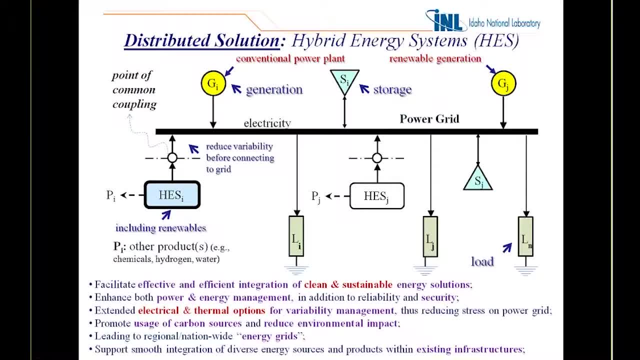 this picture to deal with our ability. now that is coming, our renewable is the intended, maybe use some level of storage there again. it could be electrical storage, it could be a thermal storage, it could be things like a pump hydrant, so forth. and the new elemental is come also to the which we are working in. is what? 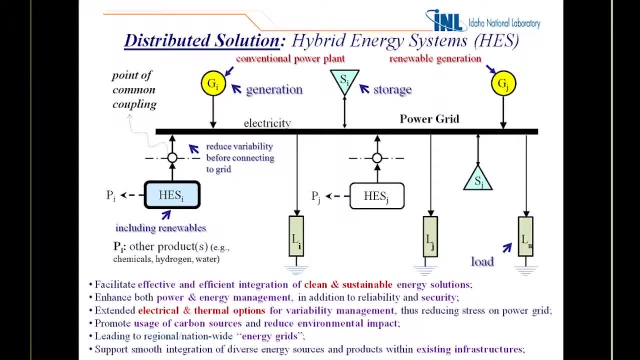 we call high rating system and hiring the city are sitting there now. kindly couple different resources with intent of trying to minimize the effect of the reliability tools or renewable, and be able to still utilize the safety infrastructure so they're not in damn a. in that way, the hiring system then, even though might have 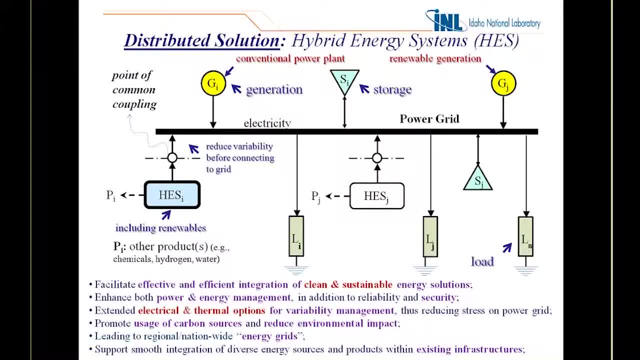 being as a dispatchable source of electricity to the grid, but at the same point it for those that might produce also other products when there is an excess of energy, and this product may be chemicals, hydrogen water and so forth. and I said we go to the presentation, you will see a little more details, who might 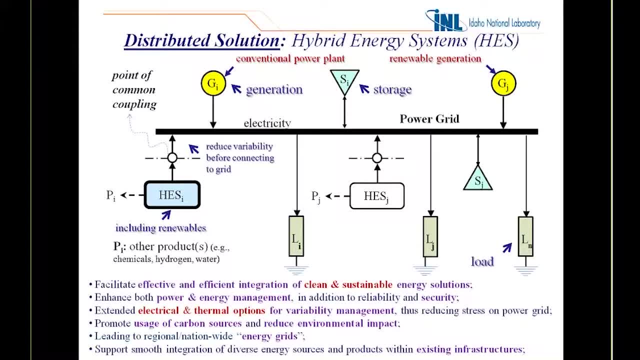 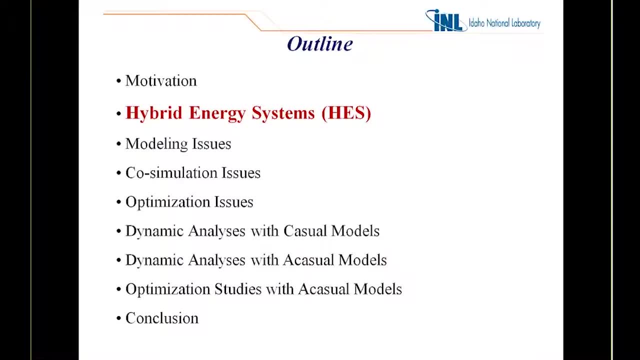 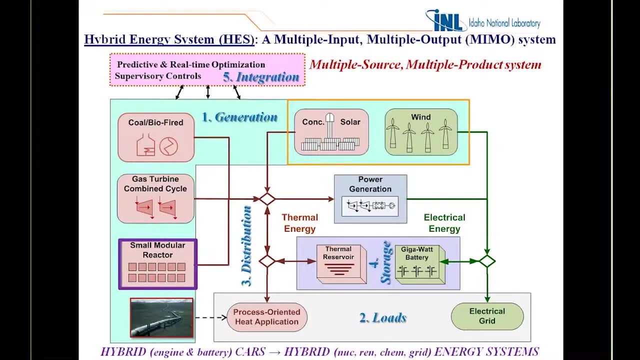 be inside of that box. I really. so that's a picture of the motivation that while working on this, and then let me, let's go into the hiring system, so I really see time. you see there, yeah, is constituted by a five different elements, so you have the generation of energy and 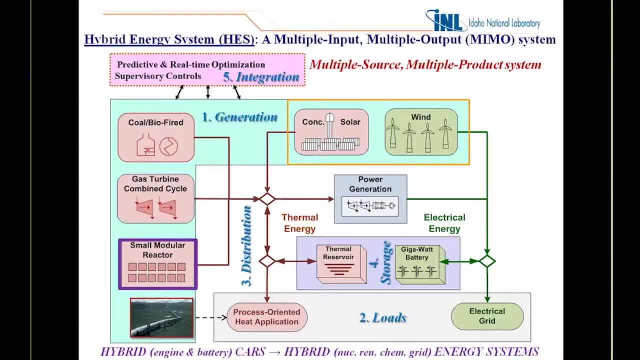 those ones. if you see to the left, my be constituted by a base lot energy sources, and you have there the gas turbine, coal, but then also because of the size in that small motor reactor on the generation, on the generations of tools. if you see to the top right, you see then renewable and renewable again could. 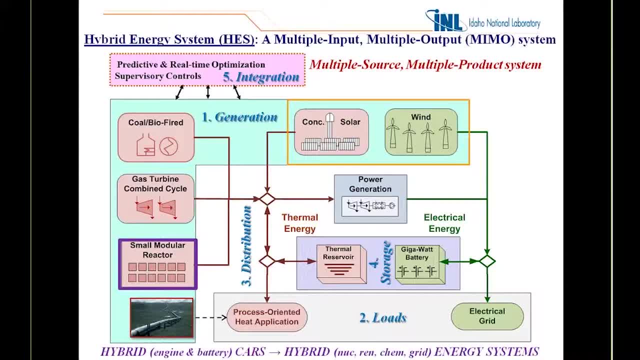 become as a form of wind, solar, many other ones anyway- then obviously we generate energy is because there is some consumer of it. so the second element there you see on the bottom, are the loads and the load it can take, the energy either as a thermal energy coming in or 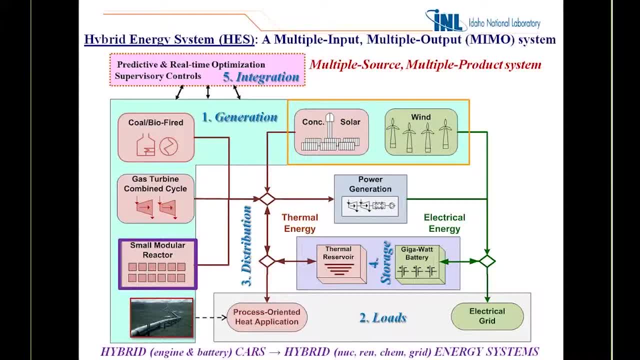 as electrical energy coming to the right, as you see there, eventually to to, to, to connect those two worlds. so we have a third element is the distribution. the distribution that allows us to again take energy generator, the generation, and put it into the loads. then the other four elements was mentioned. 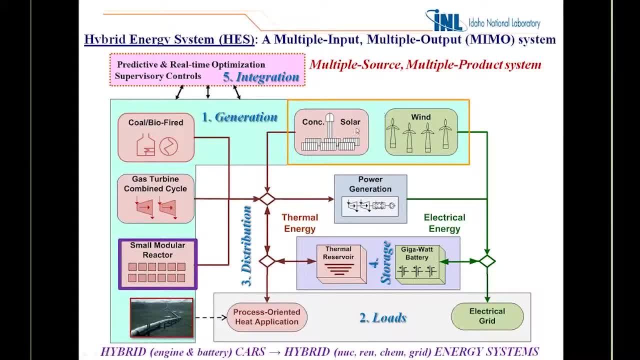 in is to deal with some this level, these viability, the DC 10 D, this energy sources introduced into a system. we might have some level or storage there, and that storage could be thermal storage or it could be also electrical storage. finally, as you see, you create a very entirely cobble system and then for 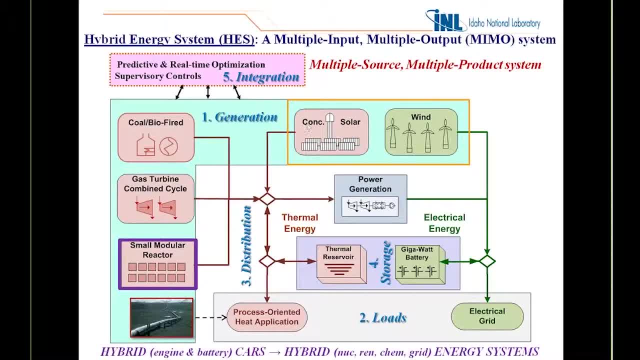 connecting them and making them to operate in a cohesive matters, that we have the integrations and then we have the energy generation. make sure that has viability introducing by the renewal generation changes and viability introduced by the loads, the integration control, monitoring controls. this function is to mobilize. 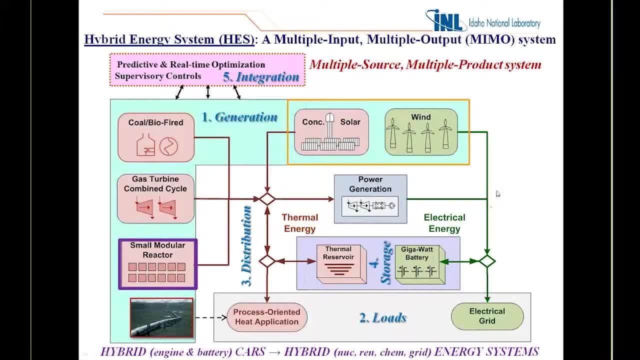 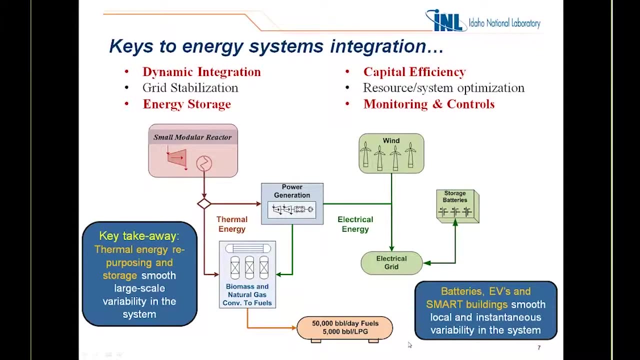 the thermal energy here and this electrical energy here, to improve efficiency in the system, resilience in the system and many other attributes. So this is like a hybrid car, but a much, much bigger scale, you might say. Or here is just to give an example of how one of those particular hybrid systems might. 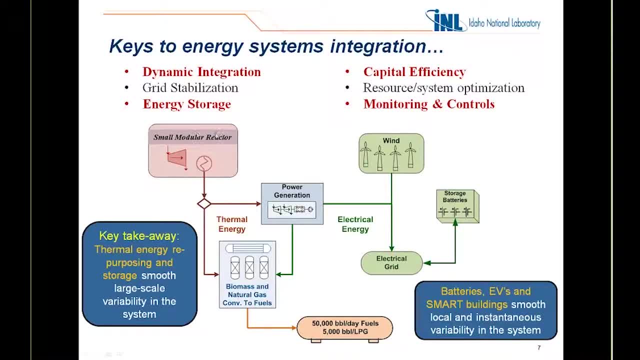 look like. Well, here you have again a generation, the base load, the small-model reactor producing out thermal energy. there And in a classical approach, you will have that energy going to the forward generation. whatever that is, could be a break-through cycle, so forth. 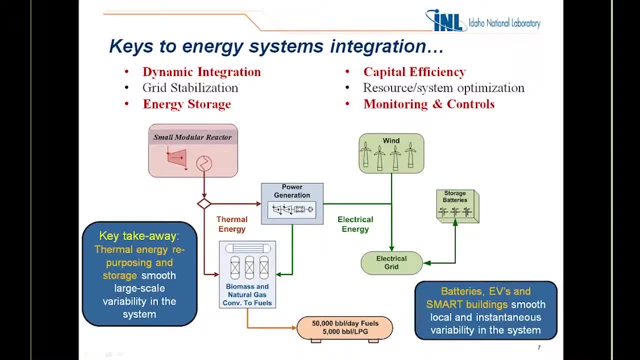 And eventually feeds the energy, The electrical grid. But if we introduce now the second element, the wind, introduce viability. so if for once we assume that the electrical load requirement is a flat one, so when this one comes in line, so there is an excess of energy, then 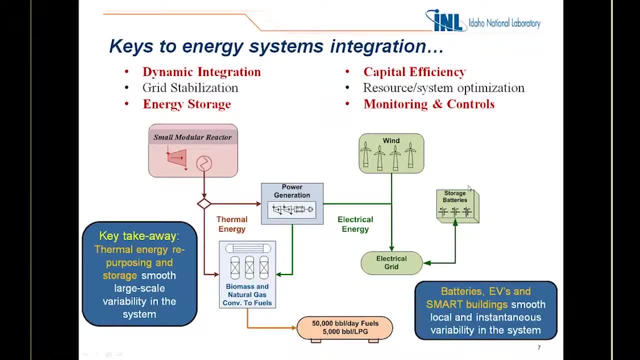 So you can manage the excess energy, either by utilizing, as I was saying, an element of storage, in this case batteries, Or by redirecting or repurposing the energy. And this energy that you, the thermal and electrical one- introduce something else there. 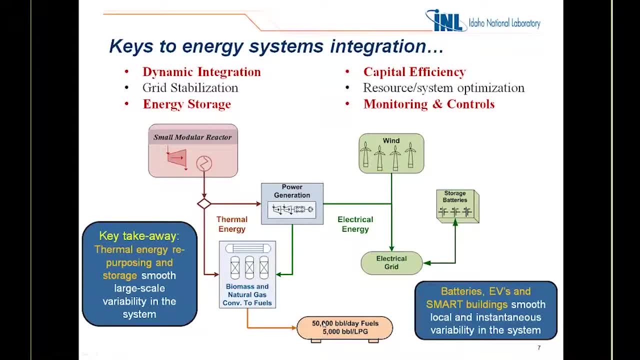 The benefit of doing such an approach is you create an extra freedom there in how to manage energy generation and utilization. So again, some of the challenges is how you do that in a dynamic matter, How you actually devise the storage in a thermal electrical. 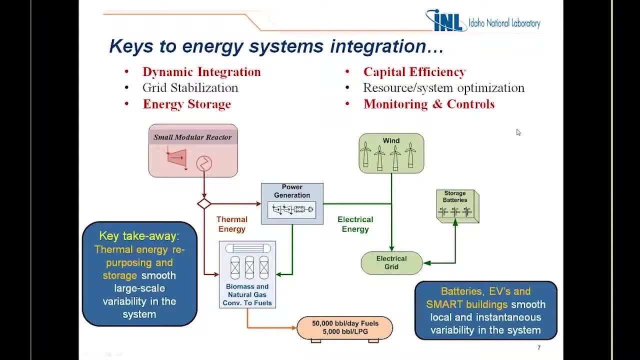 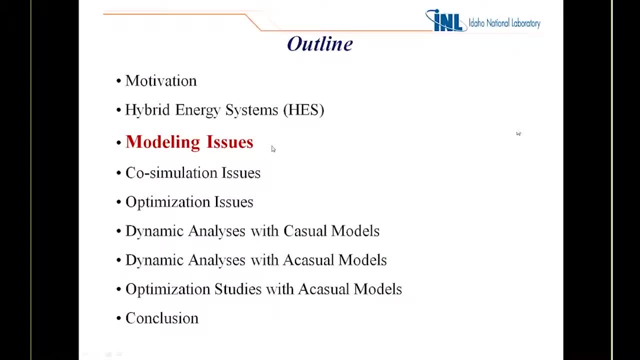 How you best maximize the capital, And then how do you do that And how eventually put all together by monitoring and control strategies. Okay, so then, and now we're going to the modeling. As I was saying, this requires a lot of innovation in all aspects. 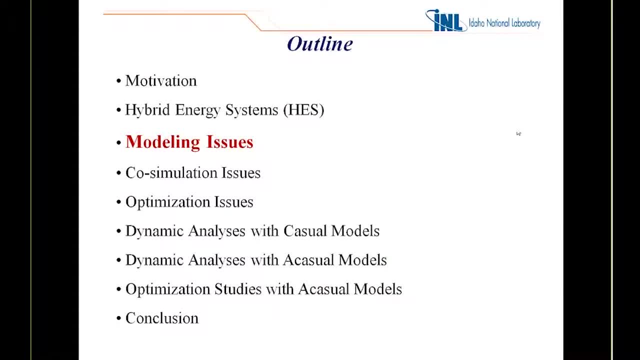 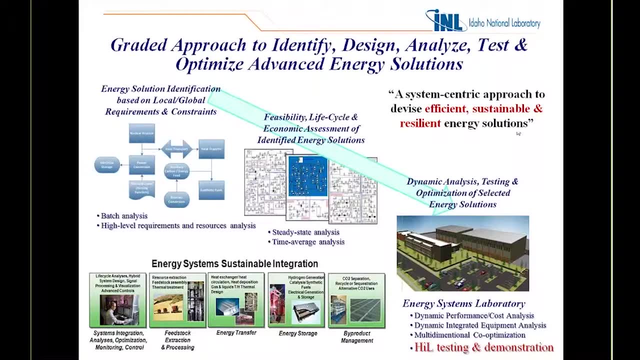 Modeling, simulation, optimization and control. So let's check out some of the things. on the modeling portion, The approach that we have here, I know, in tackling a hybrid energy system, is to doing a gridded approach in which, given a region, for example, let's assume that we have a gridded 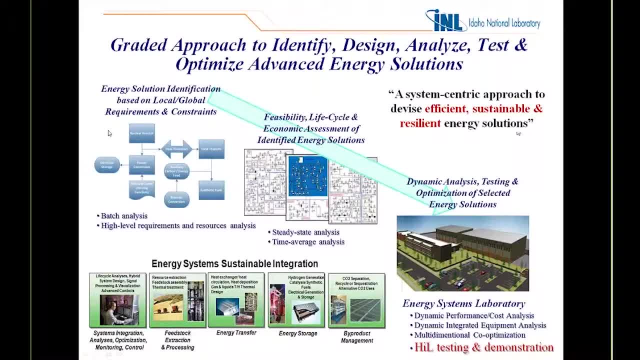 system. Let's assume that we have the western, we have Wyoming. Wyoming has some needs on better utilizing the energy resources- let's say coal, natural gas and also renewable, let's say wind. So we look into the area and do a global analysis of what kind of hybrid energy system makes 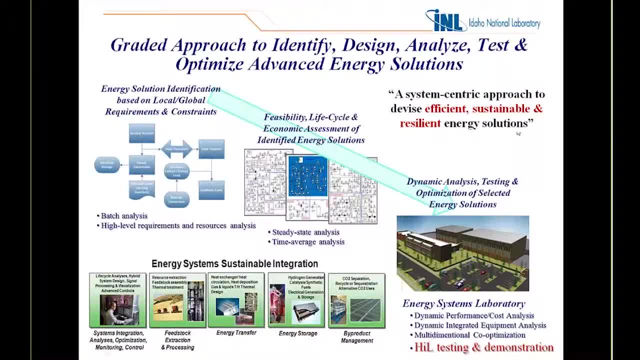 more sense there, given those resources. Given that, then we go to a level of more detail in which we do a process modeling And in this case we're trying to see: does it make sense? Does it make sense, Does it make an economic sense of what we're putting together? 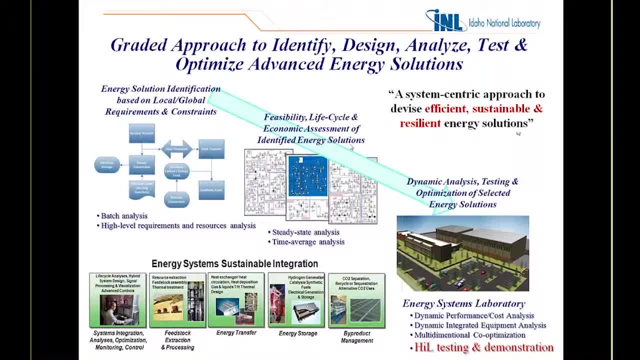 And also what kind of sizing we're talking about here, What size of the small water reactor, what size of the chemical plant and so forth. And this analysis is mostly done on the steady state of some sort of that, using tools like 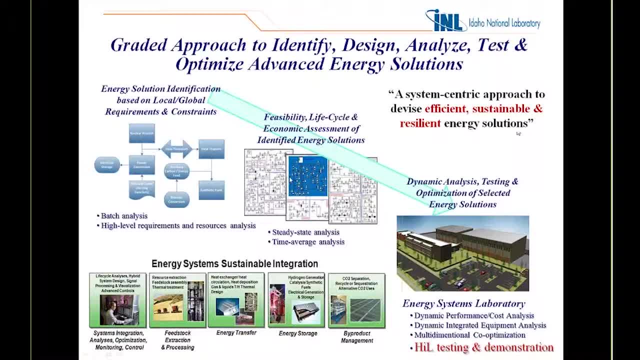 Aspen and so forth. But eventually, when we have reduced the number of candidates, then we go to doing the dynamic analysis of the system: How those different components were put together and how they can be better integrated and controlled to be able to address the viability on the regeneration and also on the consumption. 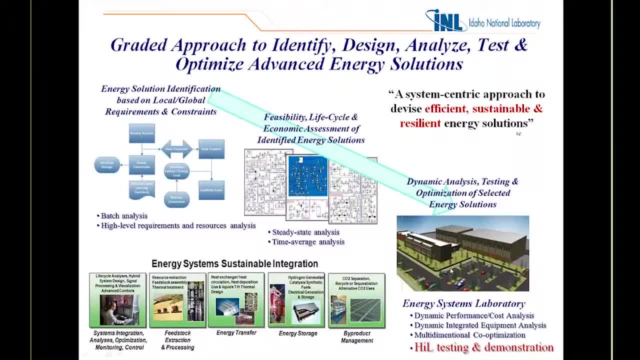 of that energy And eventually, as we do that then we push it then to even further into doing hybrid in the loop demonstration in order to minimize the risk of the plumbing of these quite advanced energy solutions. Again, I'm going very fast on this introductory. 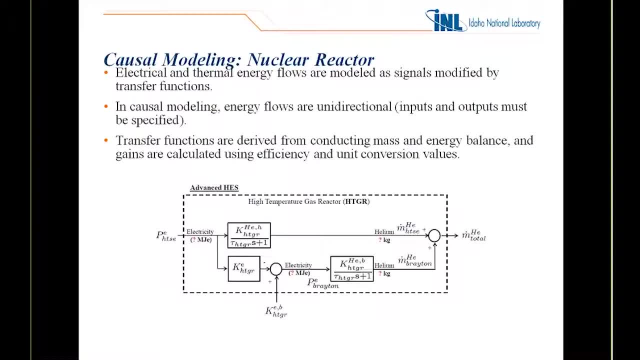 So then, also, in doing the modeling of the system, we're trying to do the dynamic analysis of the system. One might think the first one is doing what is called causal modeling. It's the one that we're most familiar with. A causal modeling is just one where you already define essentially what are the inputs to. 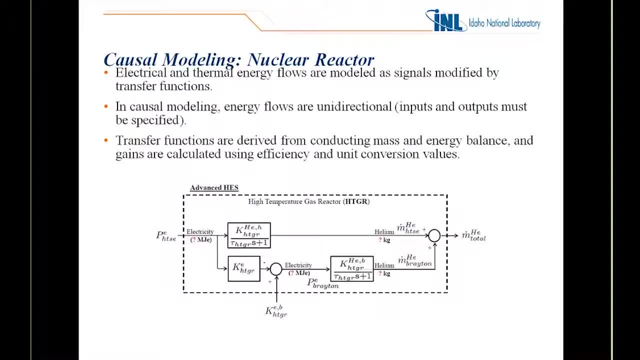 the system, what are the outputs to the system, and then you write the corresponding governing equation that deals with this energy flow. And then here's an example of, for example, a causal modeling in which we have what is inputs, the electricity. 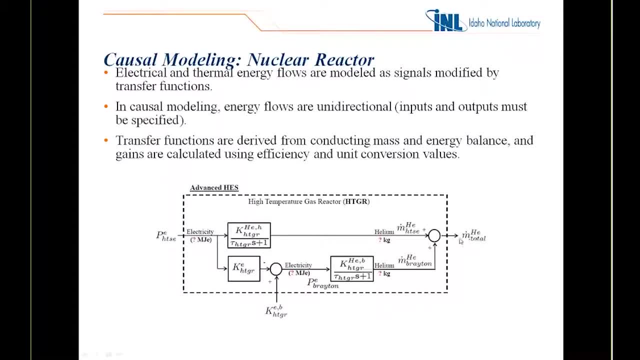 We have. what is the outputs? In this case the mass of helium that a nuclear reactor generates, both to feed a power system but also to feed, let's say, a chemical plant. But the thing here is in causal modeling, again, you know what is the input to the system. 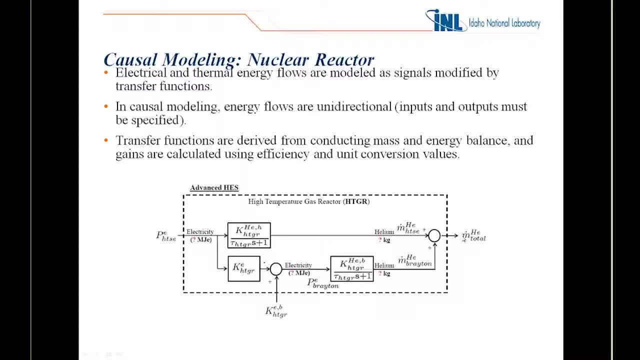 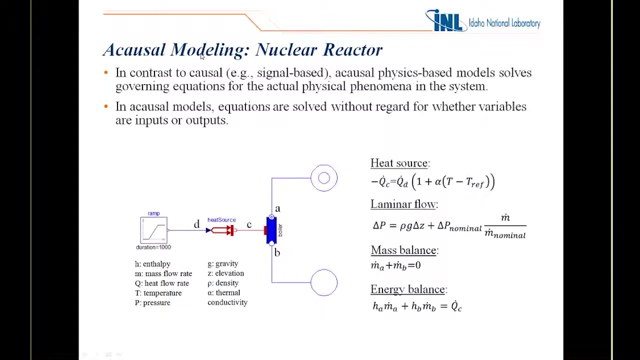 you know what is the output to the system. So in a way it restricts the possibility of the expression of energy. Hcke to ask many what-if questions. 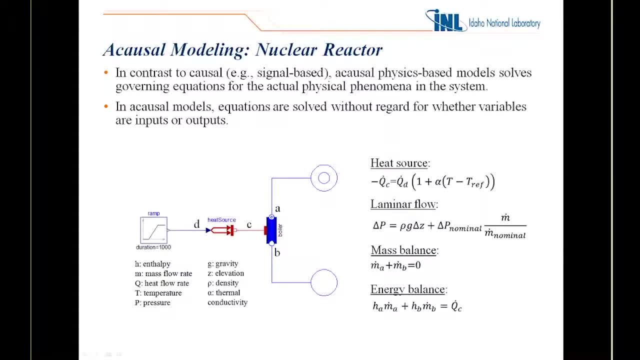 Hcke has easy answer. It's a great way to answer different very interesting questions, either by saying you can get the most creative answers, you can get the instructions Now. this is a really really fast course And also you only want to once want to have a more open kind of structure that allows. 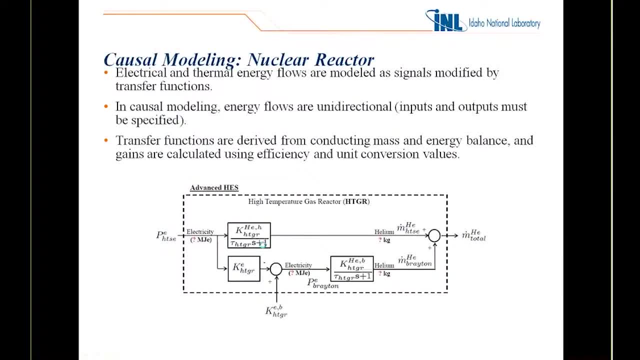 you to ask many what-if question and also allows you the usability of models, because you don't want to specify where to put the output. about that one. So I'm trying to understand this block diagram here. and so are you proposing that electricity comes in and then helium is then fed to? 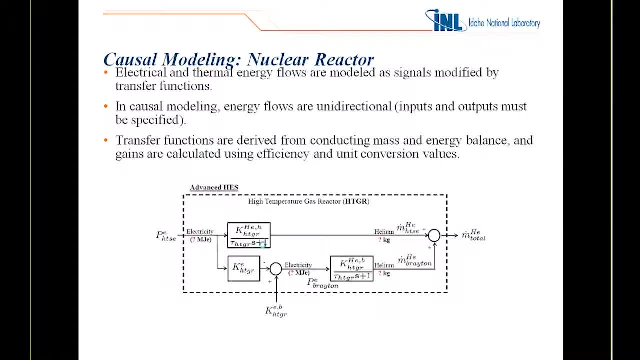 the process I'm not quite understanding. Well, you will see this particular block diagram within a bigger context, so you know what the reactor is doing here. The important thing from this diagram is that you have here transferring functions. Yes, the transfer function of the 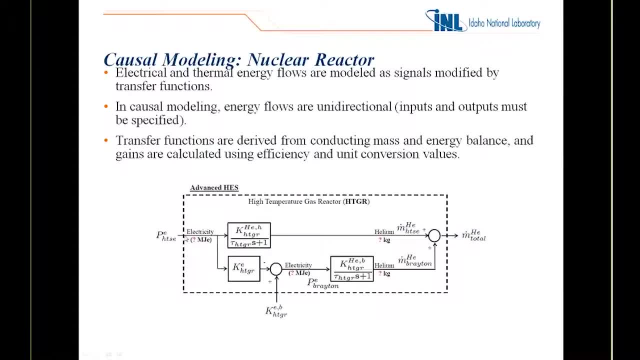 system. I think an important message here is: you define what is the input to the system and define what is the output of the system. So information flow goes this way, from the left to the right, And so this is the multi-scale modeling that you proposed in your last slide, where this is the lowest level of the dynamic. 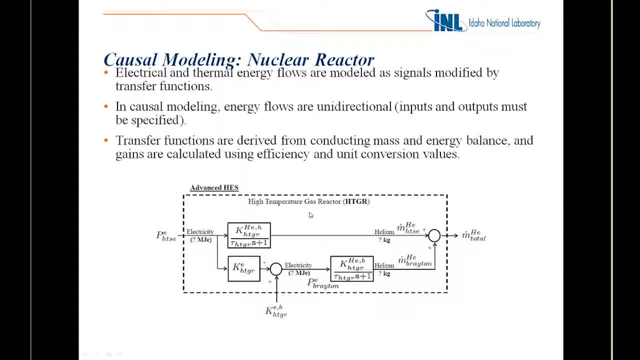 models, that you also have very larger grid scale steady-state models as well. Yeah, but also it's what we are classically has been used all the time. You have causal modeling because at the end, if you use Fortran or if you use MATLAB, whatever that is all those instructions there- they are causal. 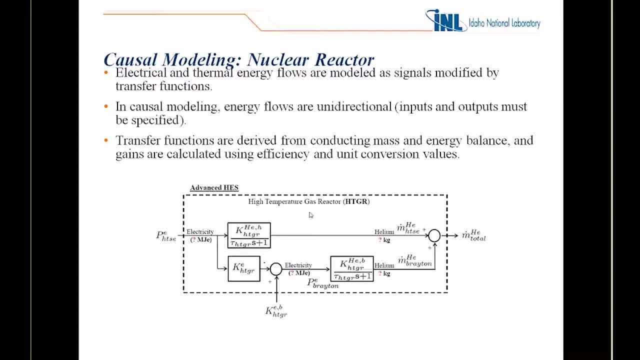 instructions there. You know what is the input, you know what is the output, But then, like I say, force you that. But in a causal modeling you actually do, truly equality of the phenomena you're trying to describe and let the system to resolve. 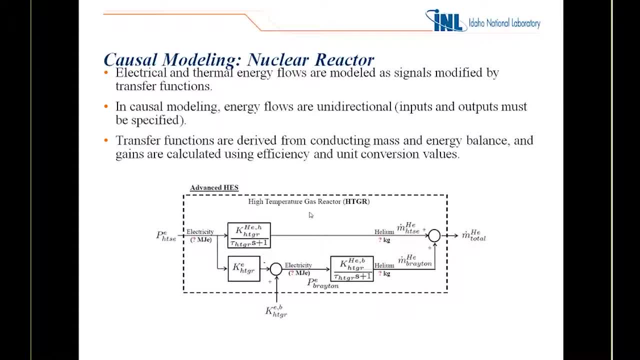 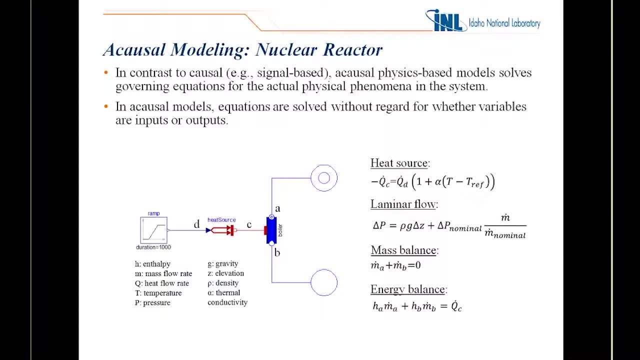 it, depending on what you're trying to do. I think it's actually a great example of where this particular model is being introduced. And, John, to answer your question specifically, you're just seeing a snapshot of an element in that larger model. This is a high temperature gas. 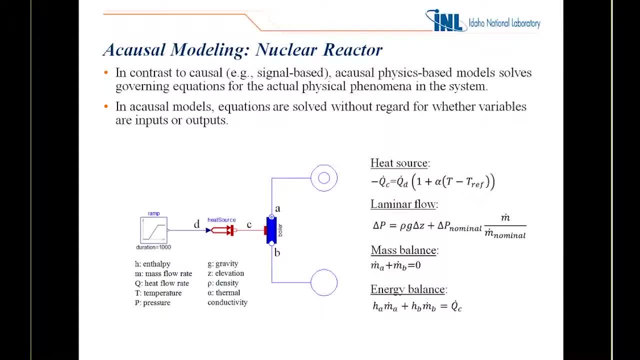 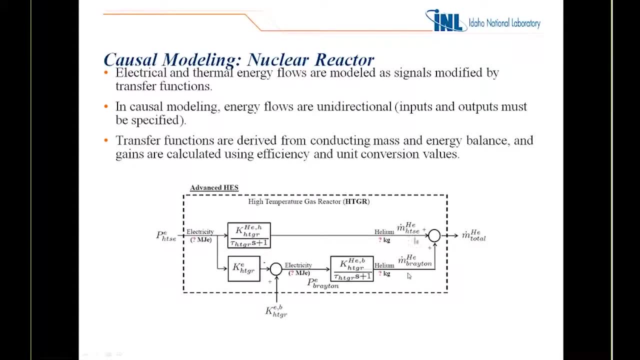 cooled reactor which is basically cooled by helium, And then that helium you see in those transfer functions is either going to a Brayton cycle to produce power, and the power is going into something called high temperature steam electrolysis to produce hydrogen. But he's just simply showing you a breakdown of 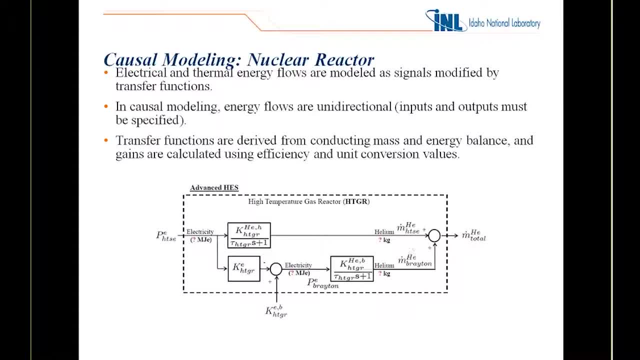 one of the elements that captures the high temperature gas reactants, which produces hot helium, and also the signal based nature of the representation of the physics in there. yeah, here you have is a helium going to the high temperatures between electrolysis and helium going through the 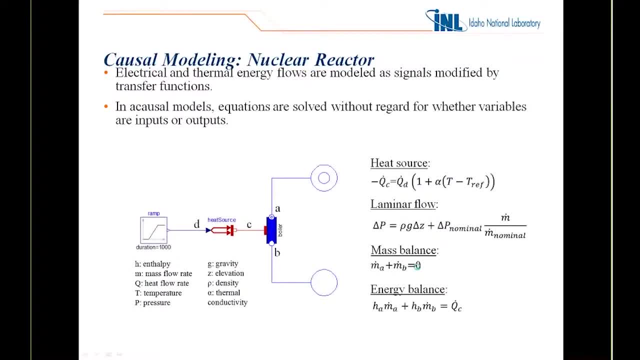 upper power generation through a Brayton cycle. now in this one, see, it passes what has been called well, called signal based, and I think great for doing control scenes of that, but actually a corrupt. it doesn't really reflect the physics that really is occurring there because he's forcing the model it to resolve the 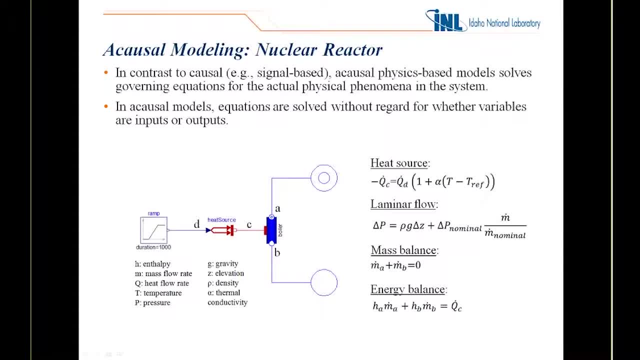 equations. so here, for example, we have a model of a nuclear reactor. this game, very simplistic is just, you know, here is a, some kind of fluid comes in, it's been heated up by this source of heat, and it comes out and are given conditions there. so to describe this system: here then we have the heat source, here we have you. 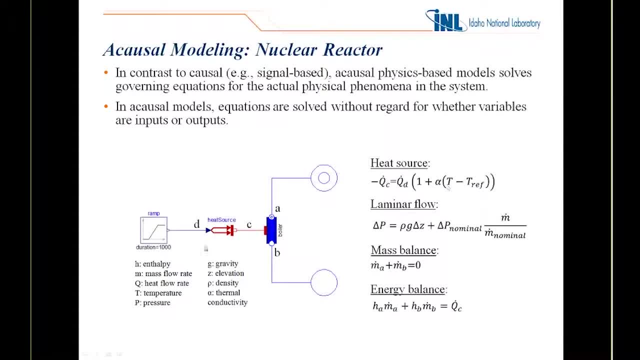 know in a way, the energy balance of it. you know a thermal energy coming in, thermal energy coming out, then over here that we have a description of the flow within this boiler. then here we have a description of here the convention: is any, any, any energy or any flow is assumed positive when it's. 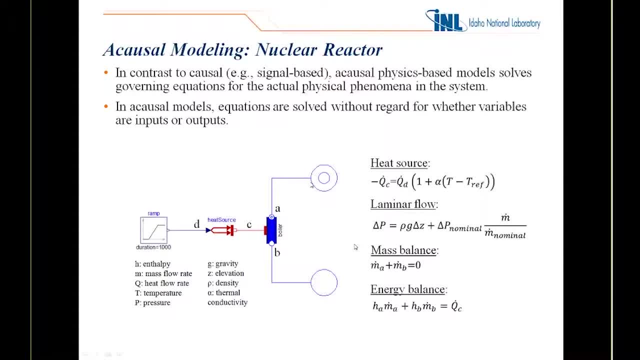 coming to the model. so then we have a mass of fluid coming into the boiler and the mass, this flow, coming into the boiler here so we have a mass balance and finally also we have an energy imbalance around the system. here you see the entropy coming in plus the one that comes in, equal the one out there now. 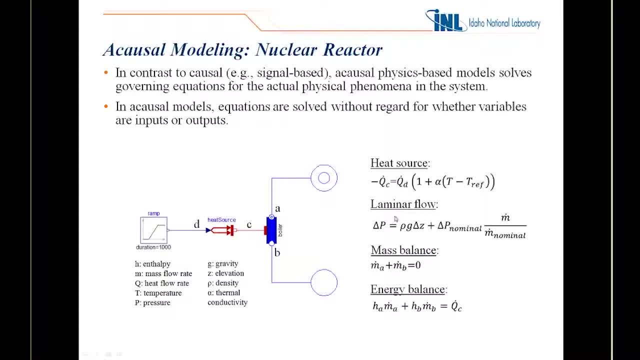 what is important here is a question is all these ones are truly inequality. you don't really say what is the input and output, so it might be that the flow goes this way: one at one point. if something changes- pressure at the free and sales, whatever it is that there, maybe they will be, maybe the flow changes and go this way. 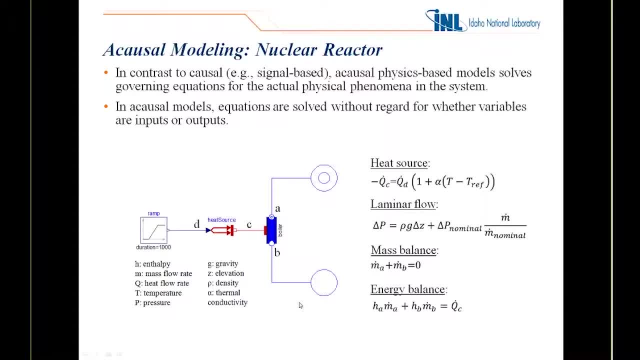 reverse of that. Well, from a modeling perspective, this is really what describes the physics, this equality, And let the computer system to resolve that, whether the flow is going this way or whether the flow is going that way, depending on particular condition of 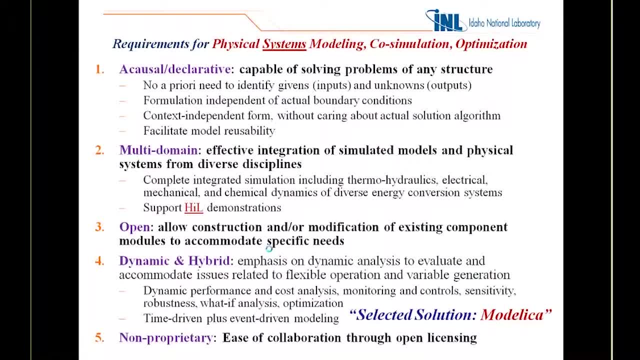 the system. Okay, so in doing that, so as we progress in the study of having a system, we recognize that we needed to have these requirements. in whatever model, whatever modeling framework we're going to utilize, We wanted to have a causal, what is called declarative modeling. 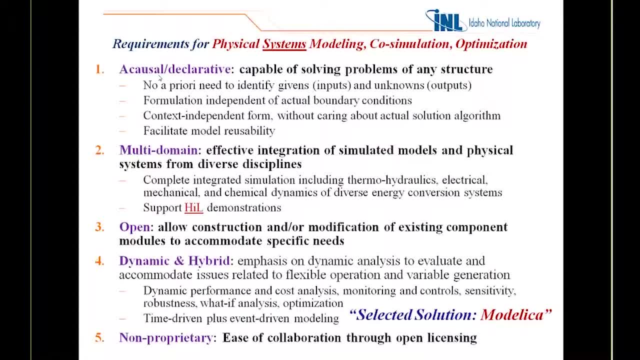 language that allow us to solve problems of any structure without we priorly defining what are the inputs and outputs. Like I said, we can go forever describing that, but that is one of the requirements that we're looking for. Then we need to be multi-domain and you will see what we're looking for. We need to be multi-domain and you will see what we're looking for. Then we need to be multi-domain and you will see what we're looking for, And so like that can be very disciplined or you're actually seeing there, We don't. 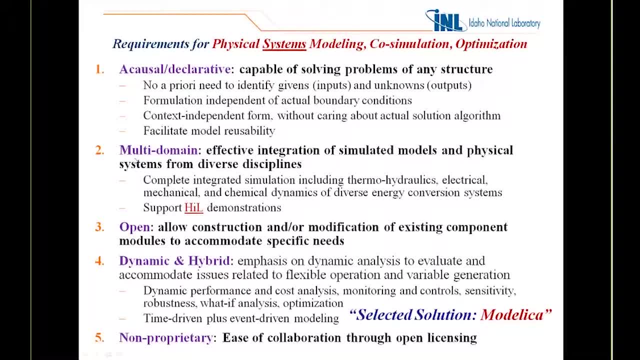 just worry about, for example, electrical systems, but we worry about chemical systems, we'll worry about mechanical systems, We won't worry about thermal systems. So there has to be an environment that is amenable to, allowed to, integrate all these different disciplines. We wanted to have it also be often there that allows the collaboration. 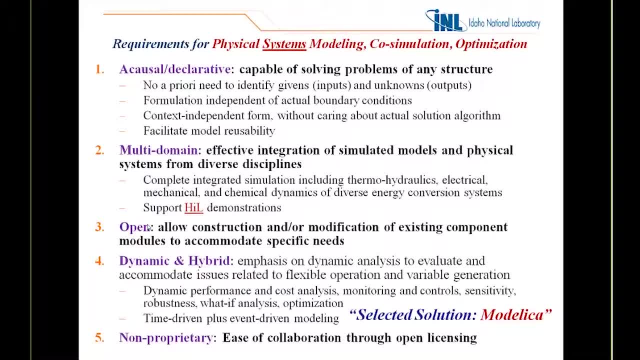 between different institutions or organizations and so forth, Because, for example, let's assume, Okay, Aspen is pretty good, but then, if you share your models with another, We're trying to do the most in the open environment, so everybody can have access to that. 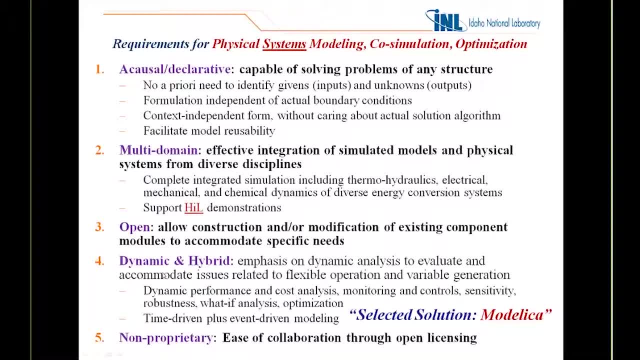 Finally, it needs to be able to. obviously, for this particular one is all the analysis that we're interested to, at least at this point- is the dynamic aspect of that. It is dynamic in only how to operate it, but also in doing the economic analysis, and so 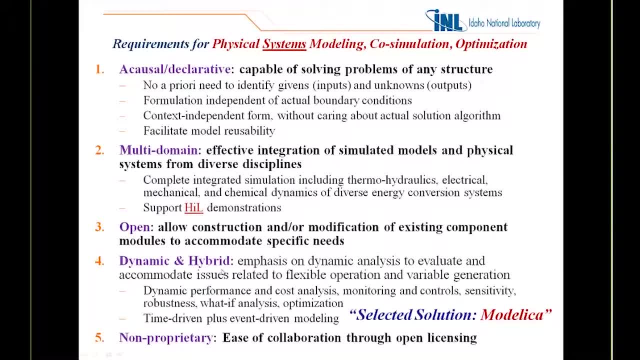 forth Hybrids. here. that means hybrid from the point of view not only on the energy, but in the same that it has time-driven dynamics, like we are used to in most physical processes, but also have event-driven dynamics. It's when you have supervisory control or seat in the react to event rather than time. 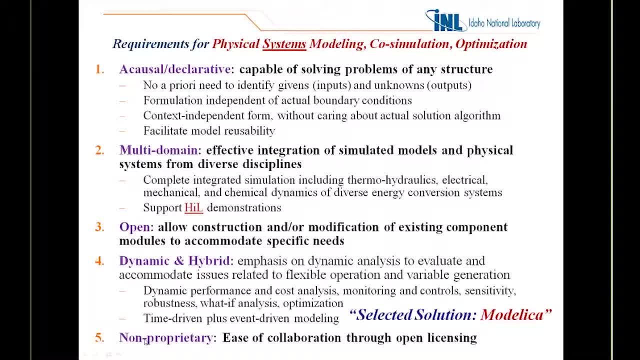 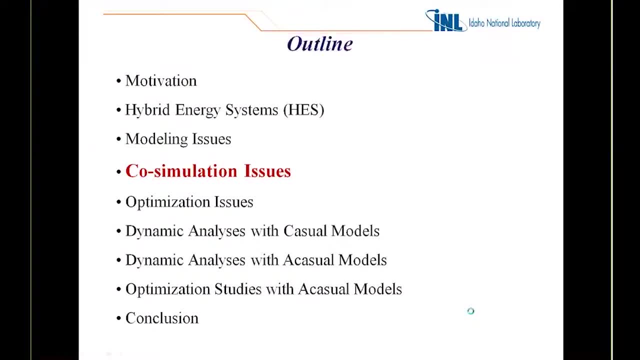 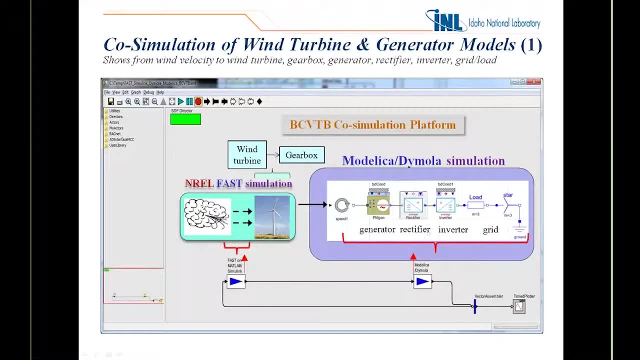 Finally, part of the open, no proprietary. so we'll use the collaboration For those particular models, whether we select Modellica as such, there are many other ones. Now the co-simulation portion of that it indicates that, Again, everyone will have a particular tool they want to serialize: Aspen, MATLAB, DICEX. 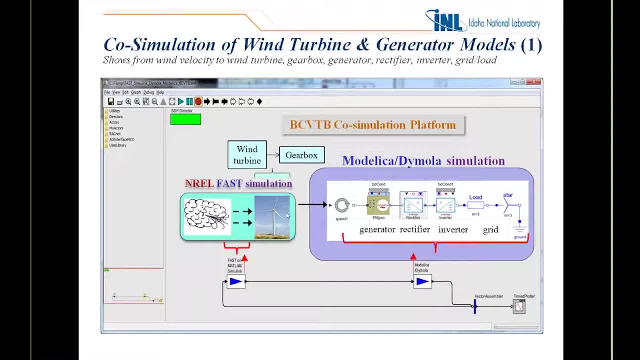 or many other ones. We need to be able to co-simulate all of them, able to put all those models some time assets together in a co-simulation so they're not to be able to emulate a much bigger system. For that we are developing a lot of tools. 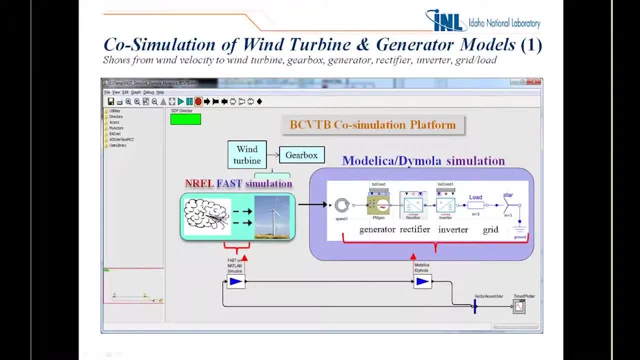 All your asset tools are already existing. Here is an example in which you have a model written in Simulink, developed by NREL, and then we have models developing in, as I mentioned, Modellica, the modeler and how you put those. 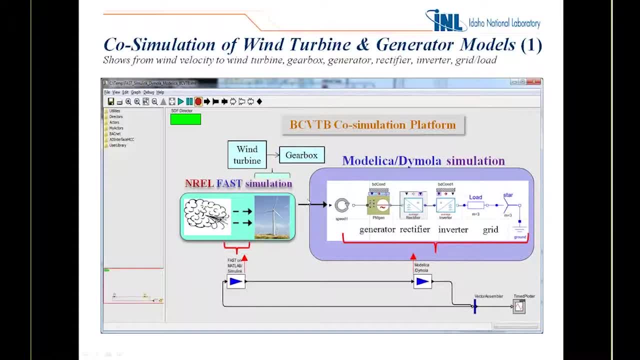 things together. For example, for that we're using this co-simulation tool, being developed by Lawrence Berkeley National Lab, but also running over PythonMate, which was developed in the University of Michigan. It's a great tool. It's a great tool. 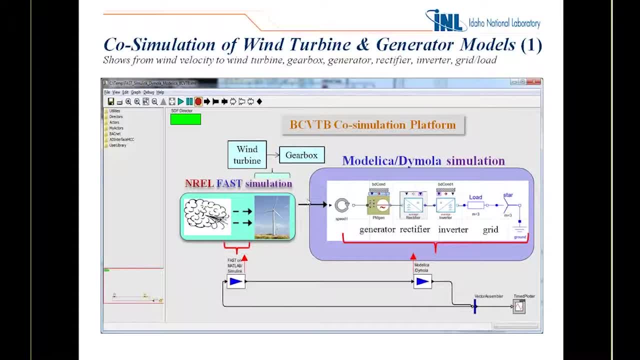 It's a great tool. It's called VCV-TV, California, Berkeley. It's called VCV-TV, which isstandbuilding control testbed. This kind of tool allows us to take models written in one environment to models written in the other environment and run all together as a much-large emulation. 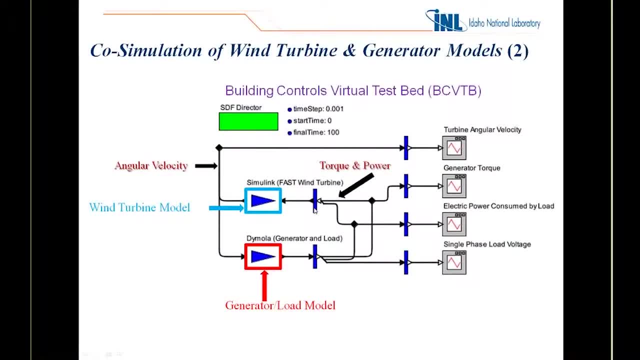 Here is how you would do it without particular tools. We are developing all the tools to be able to connect, for example, models running in in a certain operating system with models running, for example, on a real-time digital simulation. The intent is that eventually, when you're trying to emulate this very large system, 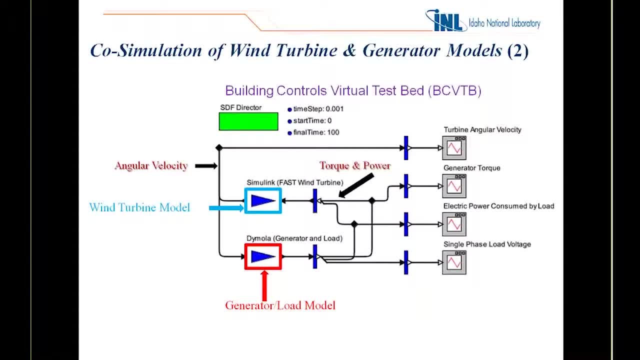 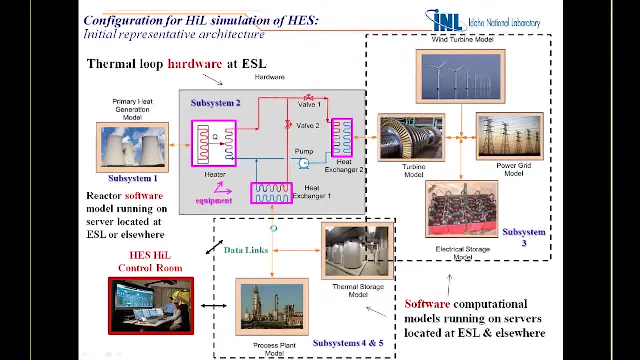 then we'll be in the need of doing some kind of simulation and eventually going through hiring the loop. This is just a more descriptive of how you would do that on this particular tool. But, as I was saying, what we intend, as we understand the system, better and better. 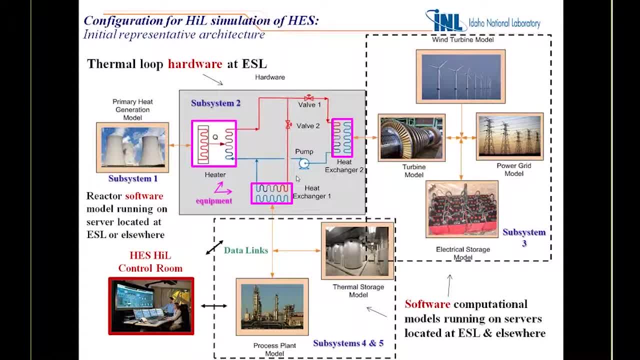 we want to utilize the unique physical assets that we have at the National Labs and create what is called hiring the loop demonstration. In this particular one, what you can see here, for example, is that, for example, you might have models of these different components, a model of a nuclear reactor. 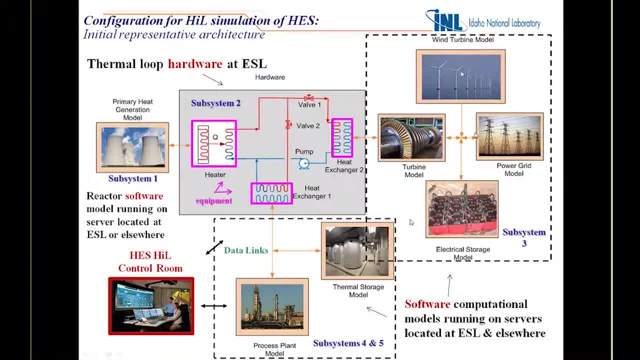 a model of a turbine and so forth and you feel comfortable that the level of granularity of this model is sufficient and accurate enough to do the analysis. But then you want to have, If the connection between them, the thermal loop, there it says: okay, how much of the? 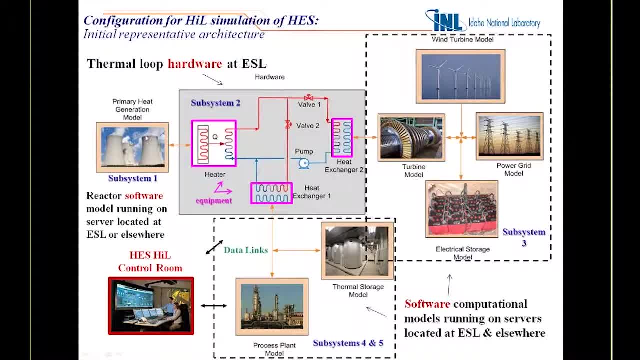 See this: The energy is generated by, for example, a nuclear and it's distributed either this way or either that way, And we have determined that that modulation or distribution of thermal energy is such that we need to have actually physical hardware connecting to that. 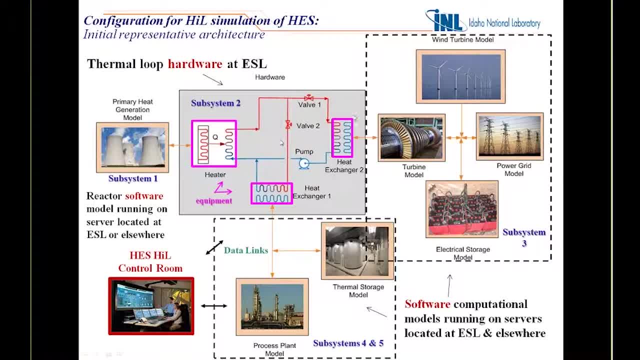 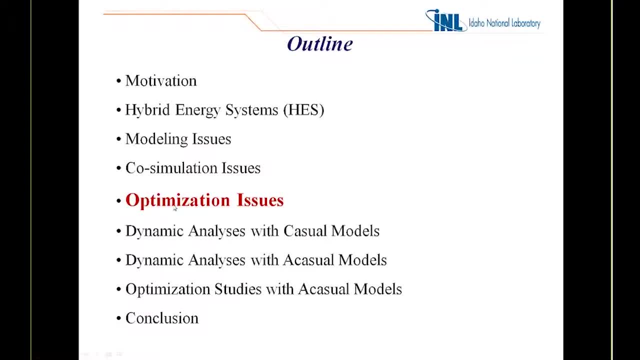 so that we connect the system, physical assets and models all together in a Connection, So simulation. So then the final issue is optimization. Again, we have to. We're doing it in how to optimize the systems when you design the system. 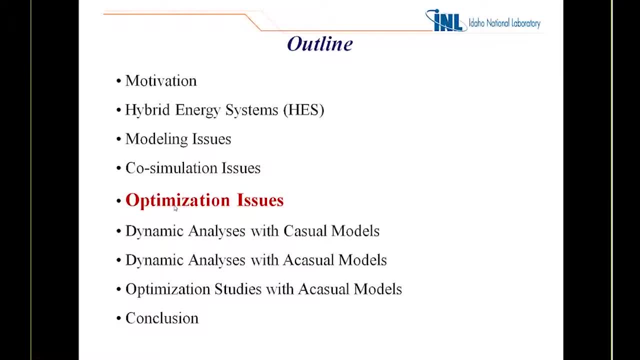 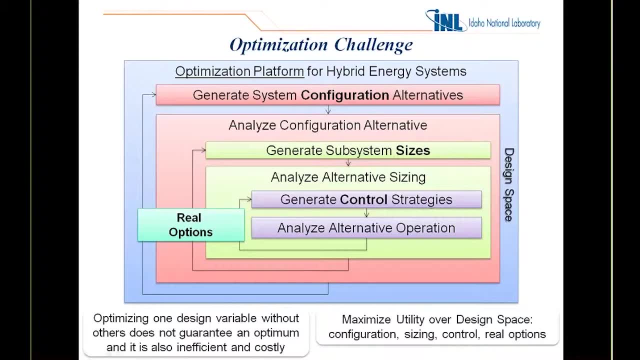 or at the same point when you operate it there. So the challenge here is: you really have a multi-loop problem here, in which initially you have to figure out what is the best configuration, given the requirements and constraints. Then, after you do that is, what are the? 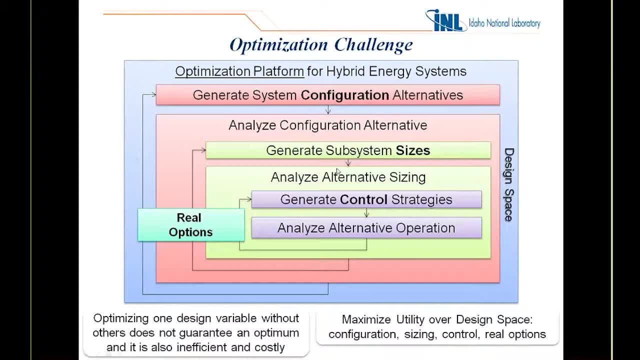 You have to figure out how to optimize of each of these components to meet whatever it needs. I mean, do they need a big battery? do they need a small battery? do they need how much of How much thermal storage is needed? how much electrical storage? 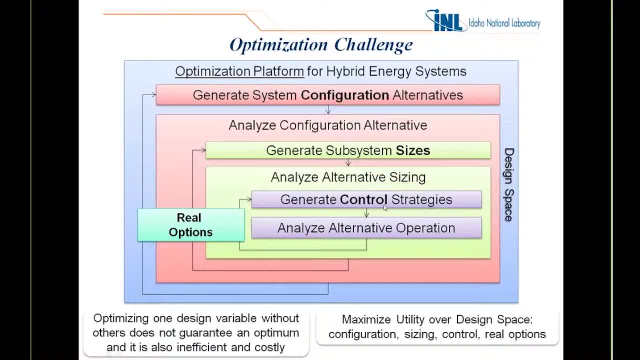 and eventually also set the controller strategy. So it's a loop within a loop within a loop. of optimization is happening there and once needs to be taken care of that. You will see some example there. There is One of the key notion here is what we call. 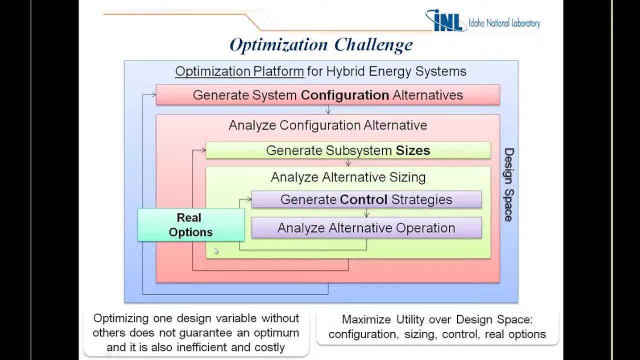 What is being called real options, and the intent is there is design system that don't have a life of, let's say, just 20 years, but have a life of many years that is able to introduce new technologies as they become available. 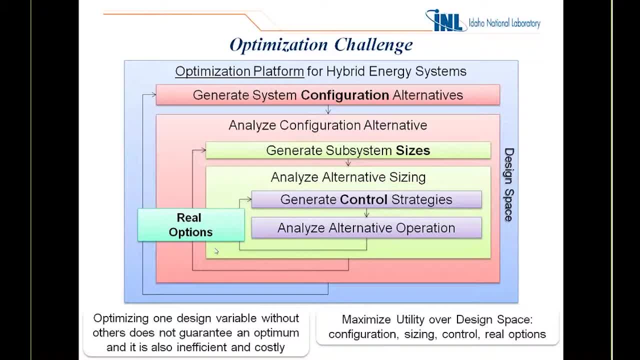 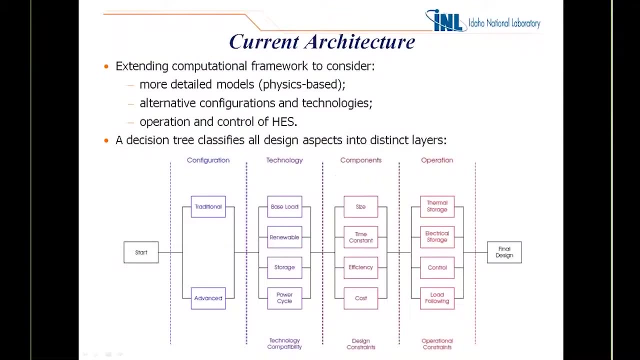 Because, for example, how many system might start using as a base load generation natural gas but naturally and easily Transformed into, for example, a nuclear reactor there? This is the big picture. this is what we're working right now. 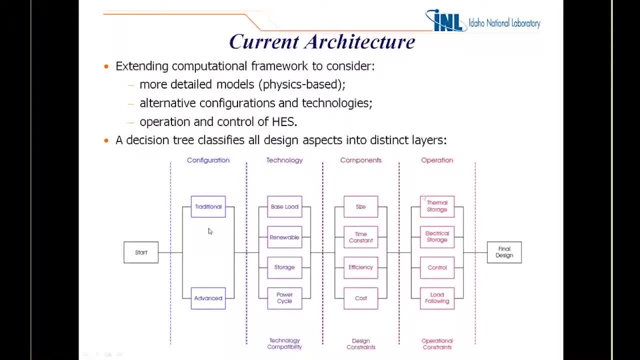 and you will see some of the result in which, then, the optimization started by saying, okay, are we going to use a traditional one, in which essentially is one generation, one load, or use an advanced, which is an energy system, depending on the requirement? 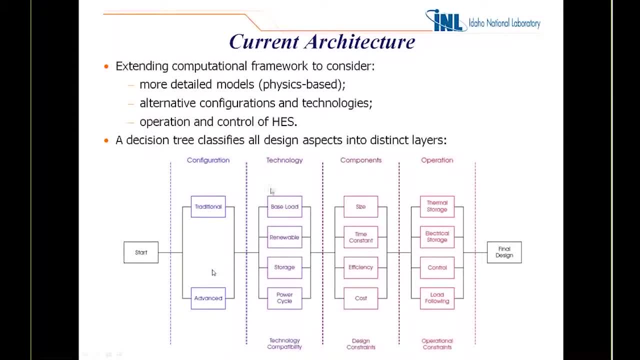 Given that, then I would say, okay, now let's select the technology there, Let's do the optimization of the technology. What will be the base load? It should be a natural gas, a nuclear reactor or renewable wind or solar, depending on the location. 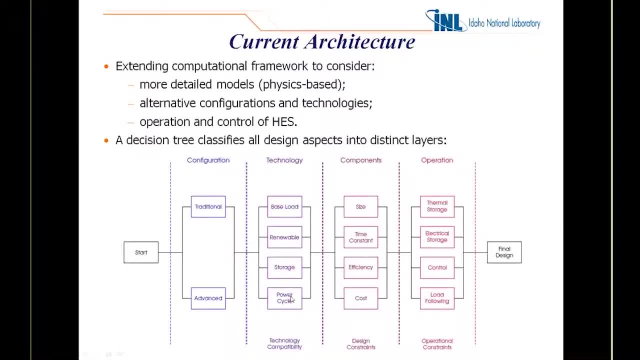 Storage- thermoelectrical- and the power cycle. It should be a Reintgen cycle or a Brayton cycle. Then you go to the next step, lower in the sizing or the size of each component, How fast the component needs to do. 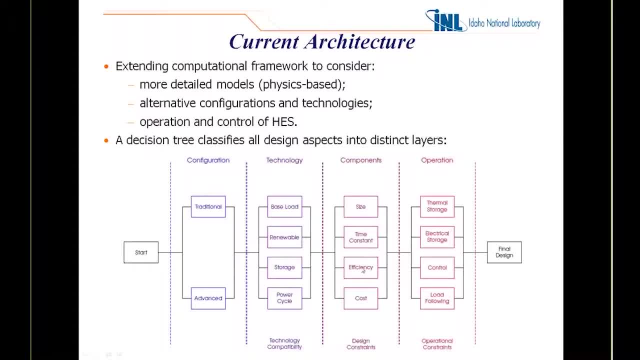 What kind of efficiency is needed? Are we okay with the molten salt a heat exchanger or a water-based A heat exchanger and the cost associated? Eventually, then, you go even further in the operation of the system. 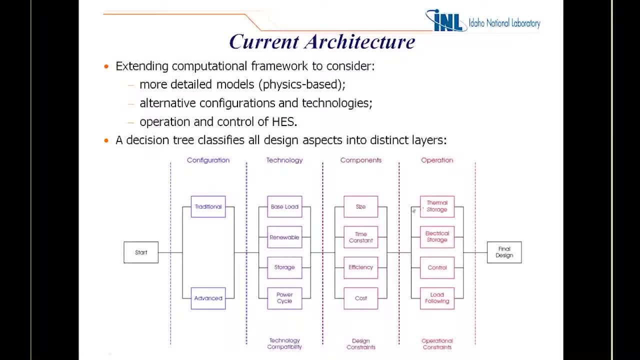 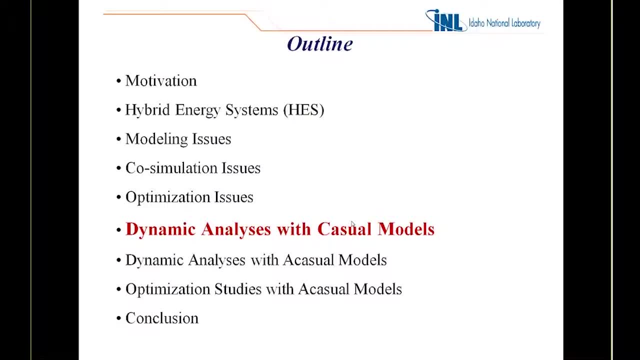 Again, you will see some example on some of those components being optimized. Then we're going to provide a few results in all two different portions of that. Okay, perfect, Then the first one. we're going to show you some of these components. 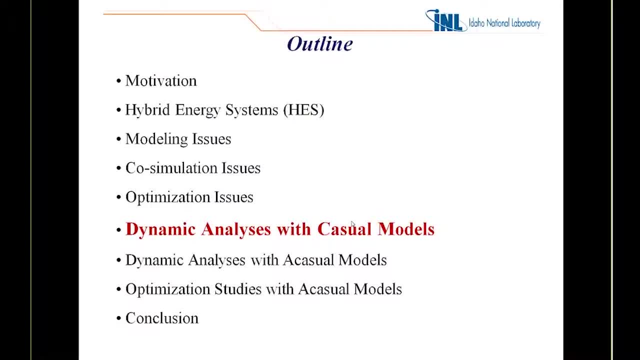 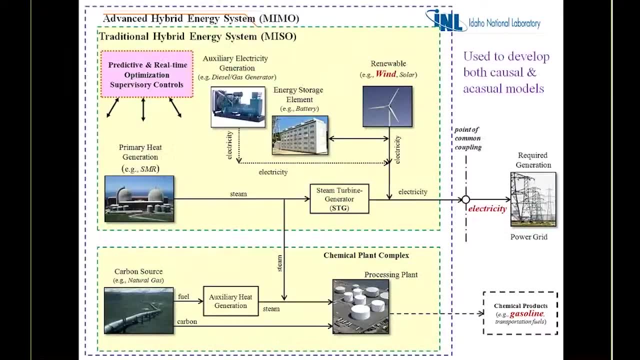 Okay, perfect, All right. Here's some of the efforts that we used using Casio models and some of the dynamic analysis on it On this one, okay, so here is. The reason we took this hybrid system in particular is because we're doing some analysis and show some promising here. 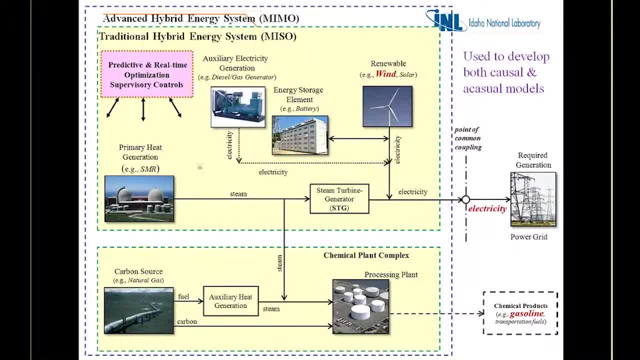 How does it work? We have a primary heat generation. in this case, a smaller reactor generates steam at a certain temperature and pressure. Then there is a steam-to-battery generation that generates electricity. Here you have essentially this: 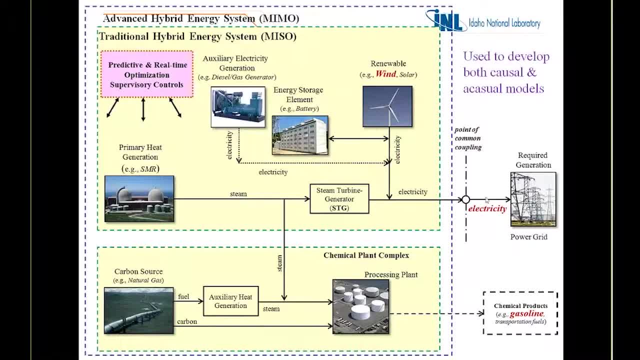 This is the classical way: One generation, one consumer. Now we include these new elements renewable. okay, so it comes in here, If you assume that this requires a flat load to here or generation. so when this guy comes in, which is uncontrollable and very variable, so we might need to have a storage here. 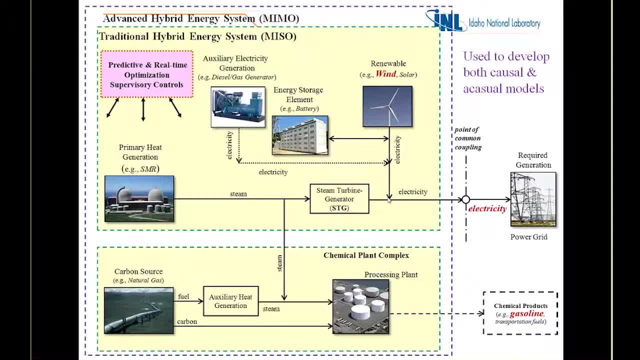 Okay, Now another approach, Oh, Another complementary approach, is: when this energy comes in here, we'll take the extra energy that is not required here anymore and send it down here to take the carbon source coming from natural gas and transform that into the chemical product, in this case gasoline. 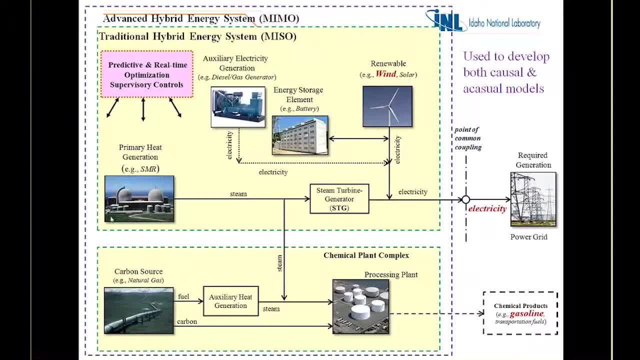 So what we did is we put all this configuration using. Actually, we used the configuration, both Models. We used the configuration using a causal model for different intents, and you will see that the best one to analyze the dynamic portion is using a causal model. 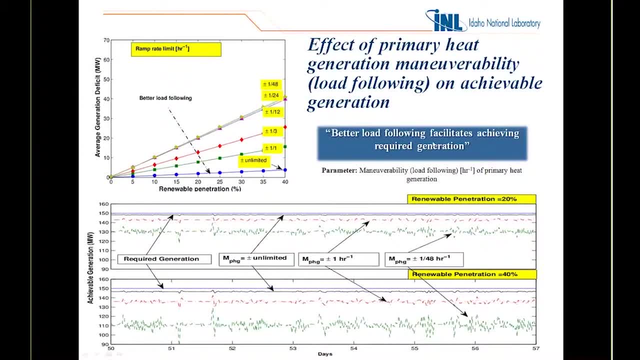 Okay, so here's some of the results that we have when we put that together. and again, it's because we want to see how changing different dynamic properties of different components change the overall performance of the system. and here's one that indicates, for example: 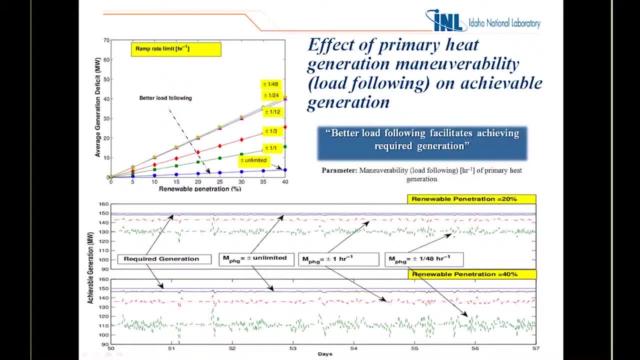 if you have the renewal penetration here and you have the average generation deficit, meaning the deficit is what the grid wants and the difference between what the grid wants and what the hybrid energy can actually deliver. So it shows that a decrease in there. as you see here the deficit, it keeps reducing. 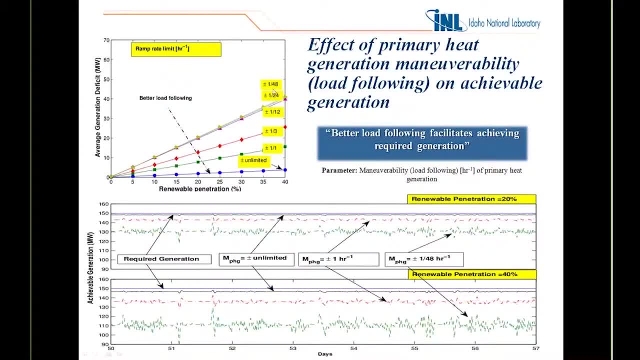 right, Okay, So this is making a system slow to much faster and faster and faster As the renewal increases. so the ones won't require the base load generation to have a better dynamic characteristic to be able to load. follow the generation and the loads. 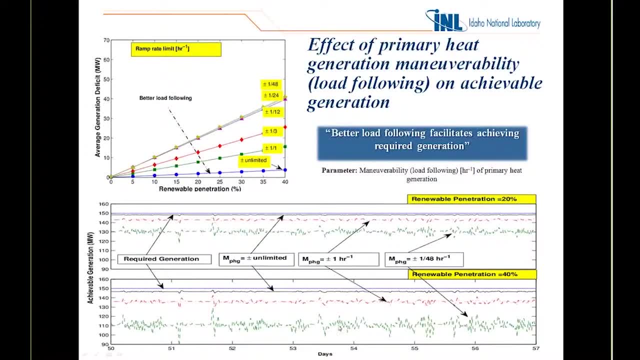 Here you see, for example, how it's a time series analysis in which here is what you want to generate: Okay. Okay, So you can see that the load follow base generation fast enough, you can get very close to it. but as this guy becomes slower and slower, then there is more deficit in what you can. 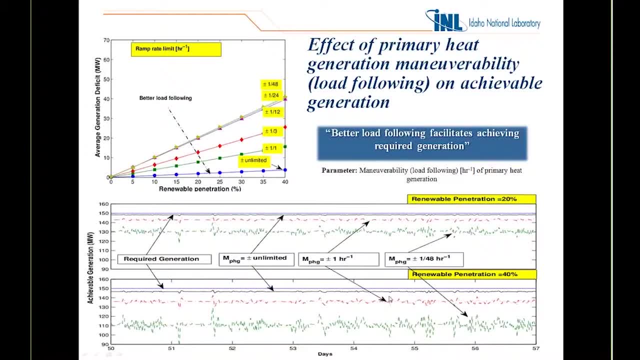 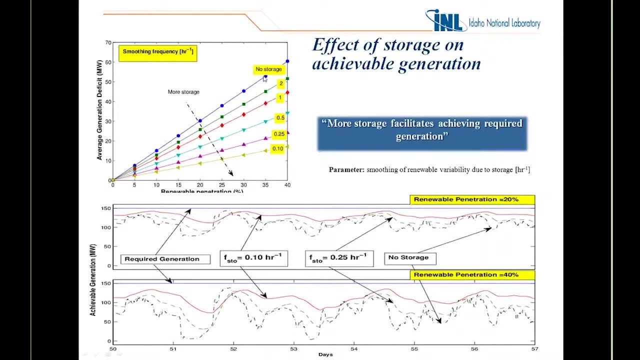 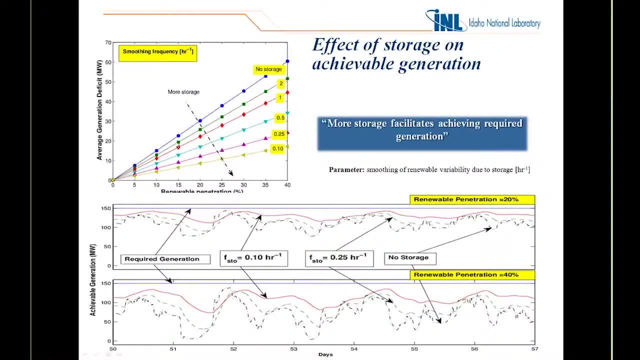 more storage. So you see here that has, for example, for a particular renewal generation. as you increase the storage here the deficit decreases. And here is, for example, how you see it in time series. Here's what you want to generate, and here is with a lot of storage, less storage and 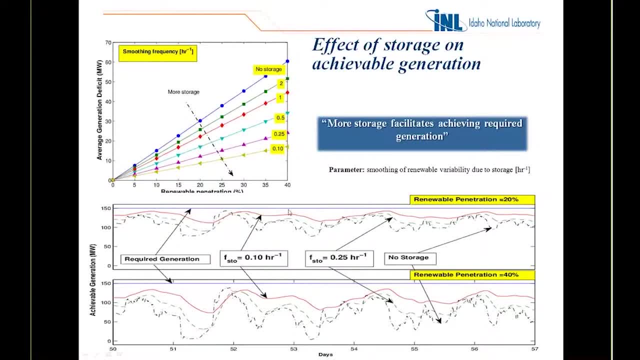 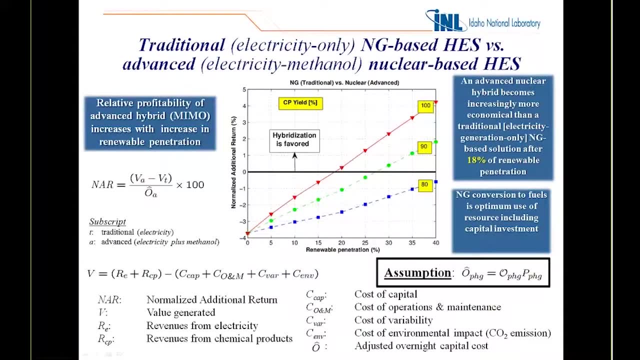 less storage. so you can see, the deficiency increases as the storage decreases. Here then again the Okay Okay, Okay, Okay, Yeah. So I think the message of this is again: here you'll renewal penetrations and here 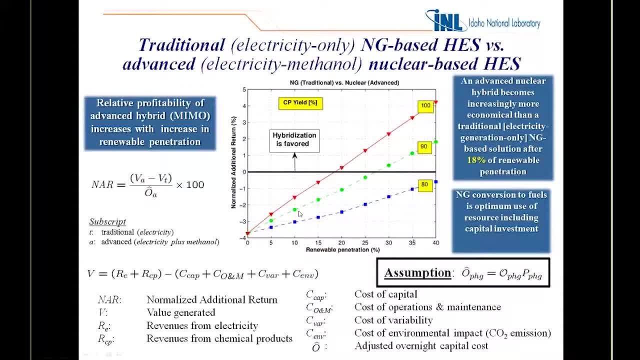 is what we call the normalized average return. This is just comparing of what is the benefits of high realization, as opposed of just taking a single generation source to a single community generation. What this system shows- All these analyses, by the way, was done in dynamic context- was this plot shows that? 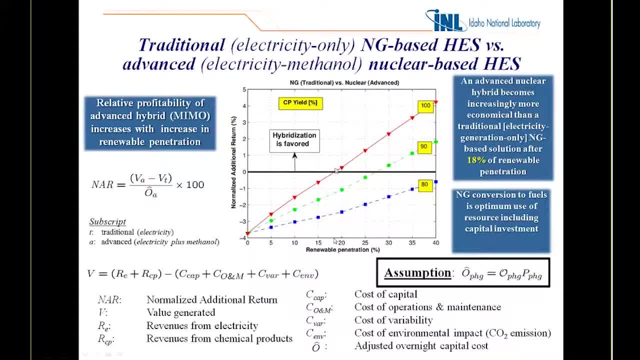 when your shift is 18% renewal generation. right here then it is: hybridization is favored, even though you- and here's compared, by the way- a national gas with a nuclear, So even though using a high capital acid as a nuclear reactor as your base load. this 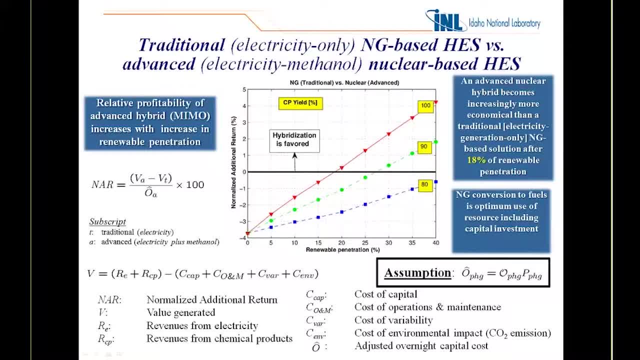 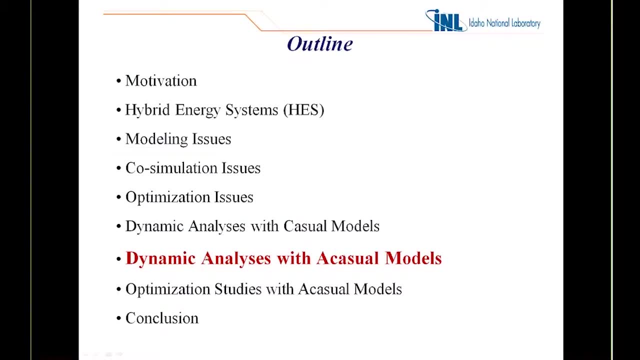 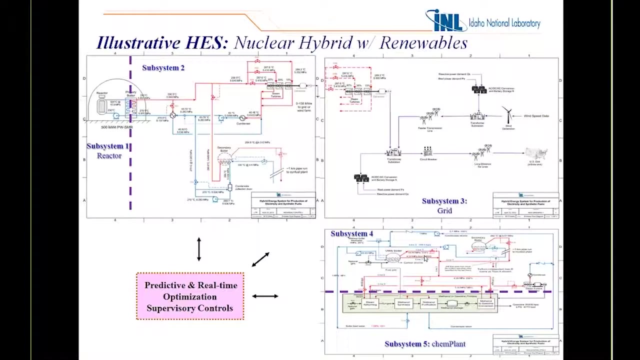 plot says that even that point, after 18%, it becomes economical to start using a nuclear reactor that is providing both electricity and also chemical product. Then now let's go and do some dynamic analysis with a course of models. So then what we did- one is what we did- was: then we took the. let me just go. 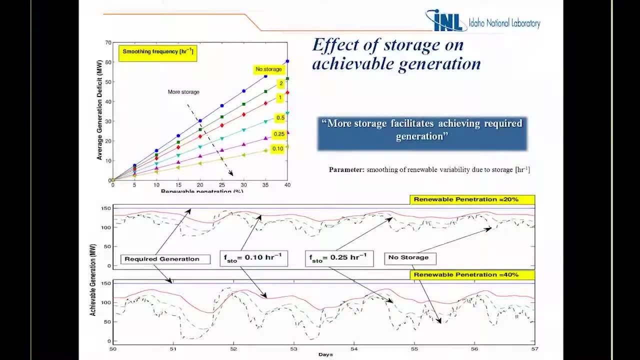 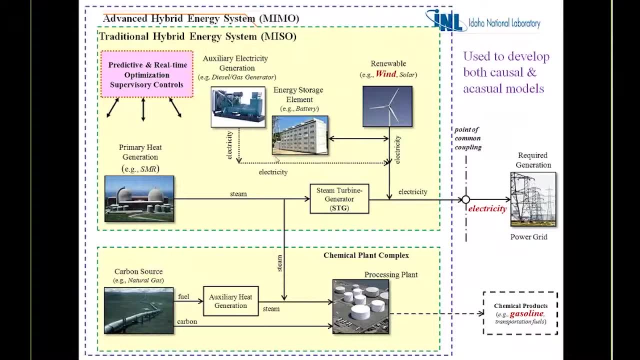 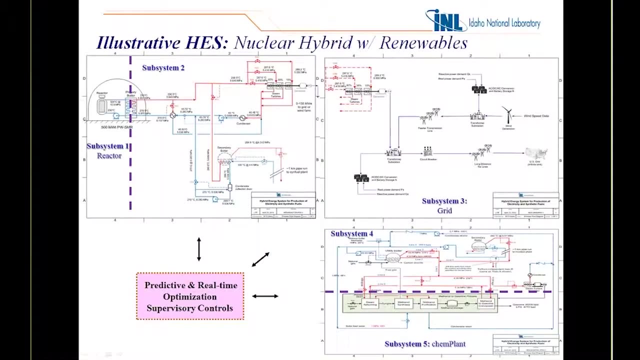 real quick. we took this one American, much, much refined or high granularity model of it, using a quasi-model. The first thing we did is: here is the safety, Here's your reactor. This is the first path And from this point it's going to the electrical grid. 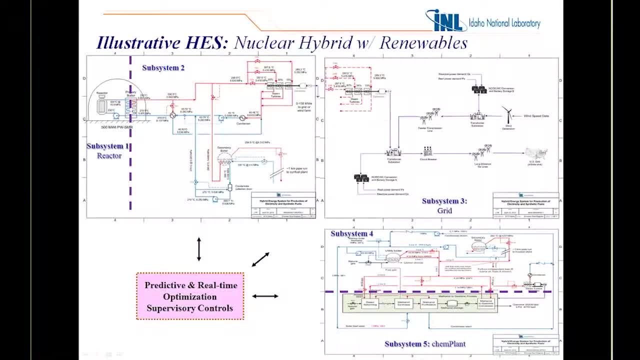 And here you have the renewable support. So normally you go this way, And now we have this secondary path, in which now the excess of energy might go this way here and eventually go this way and eventually goes here and eventually feeds a chemical plant. 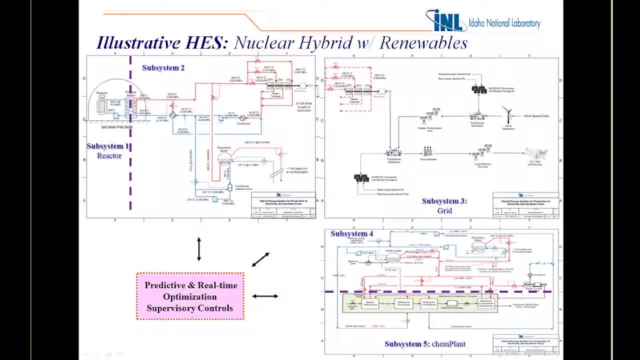 So now you see, here is a very detailed model in which now you have not only the nuclear reactor, but you have pipes, you have heat exchangers, condensers, turbines, the whole thing there, Well, complexity, and then you have to model the system. 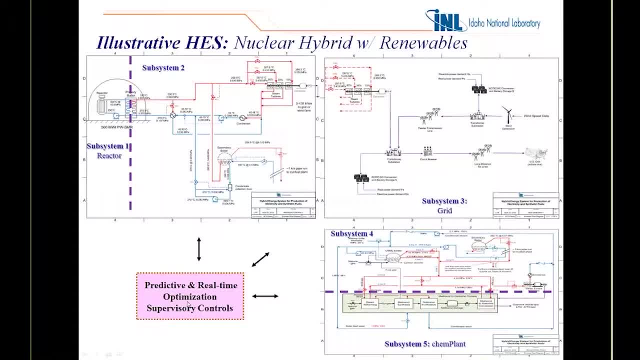 and also, at the same point, do the controls to be able to operate it there. So, then, what we did is we pulled this model first in Aspen just to do the sizing of the equipment, And after we have this sizing of the equipment, then we move into the Modelica regime. 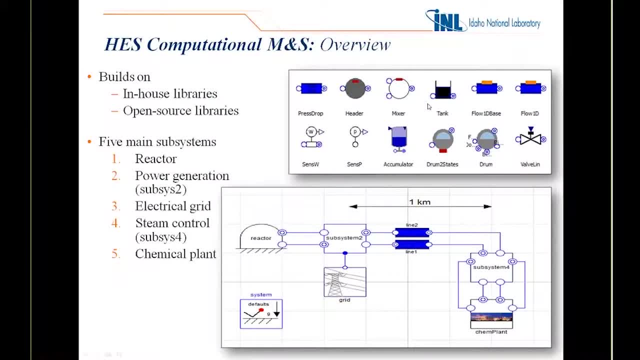 And here is the model written now on the Modelica framework, using Dymola as the tool on doing this stuff. So in doing that, so here you have again a reactor, Then it's subsisting and subsisting here And modulate essentially either some of that. 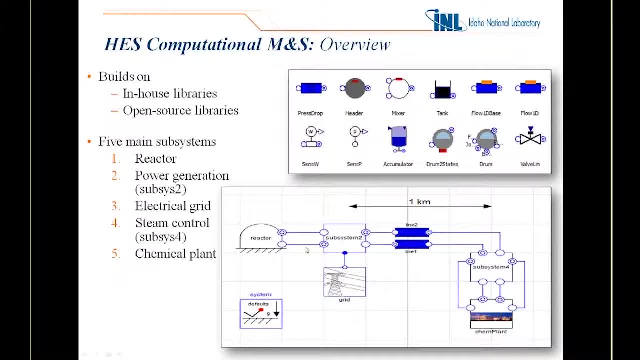 goes to electrical, Some of this energy goes, Some of that goes to electricity production, Or some of that one eventually fits and is used for chemical production, And in doing this model then we construct a lot of different sub-models of different components. 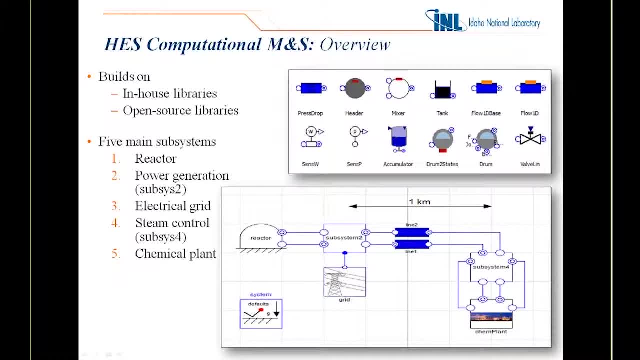 the headers, the mixers, accumulators and so forth. And the exciting part of those things is that all these ones again were a causal model. So allow us to easily reuse those models in many other configurations without constraining ourselves. 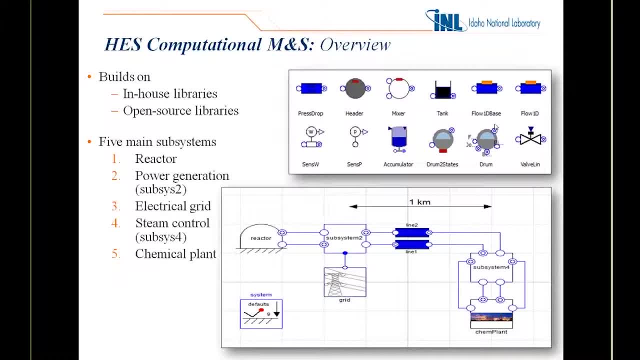 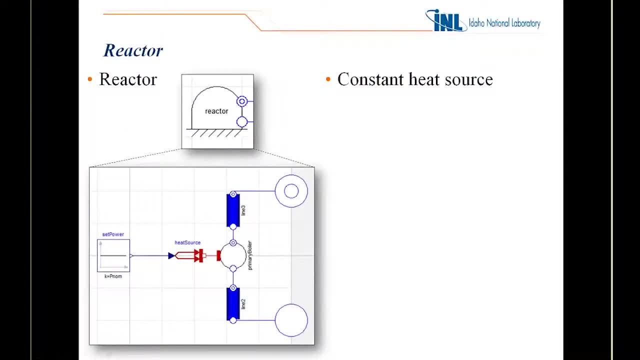 in the particular configuration that we eventually will use. All right, so then. so, just briefly, again is, here is the model of the reactor. In this case it was very simplistic. We have a much, much detailed one of it. 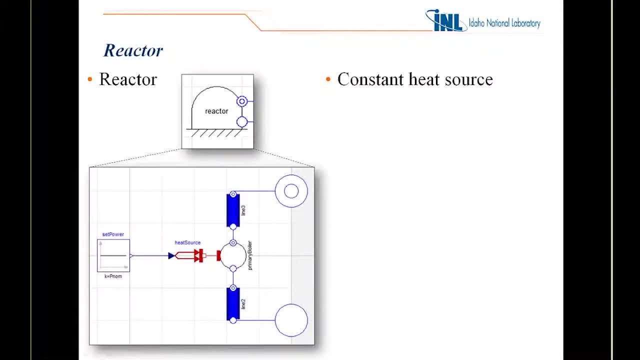 But just for the presentation here to show you, it's essentially a heat source that heats water coming in in this fashion And, as you see here, it's essentially assuming that the reactor is in a certain operating condition And then it just go and heat it there. 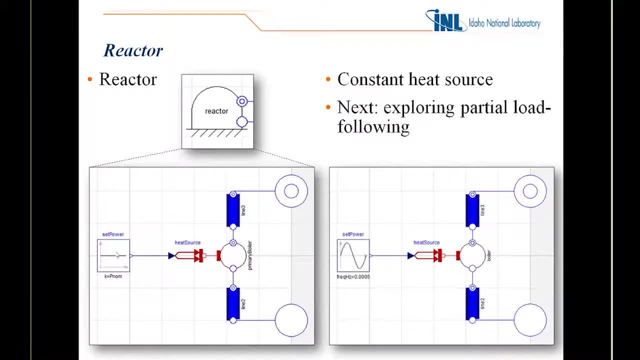 Here is similar to this one. The only difference here is allows them now to low-follow the reactor depending how it changes on the generation of the renewable and changes on the markets there on the other side, And see the benefits of low-following at the generation side to meet the electrical demands. 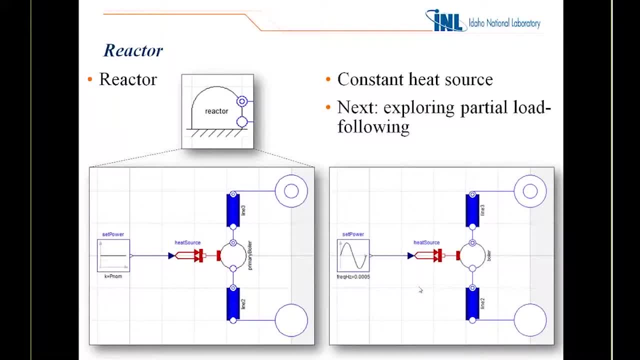 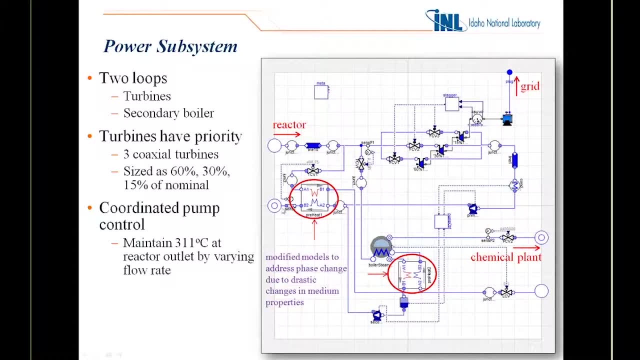 or the chemical demand, whatever that is, Thank you. Here is going then further on into the model, And here you see, here will be the reactor. Here is whatever is producing is going to the grid. Here is whatever is producing going to the chemical plant. 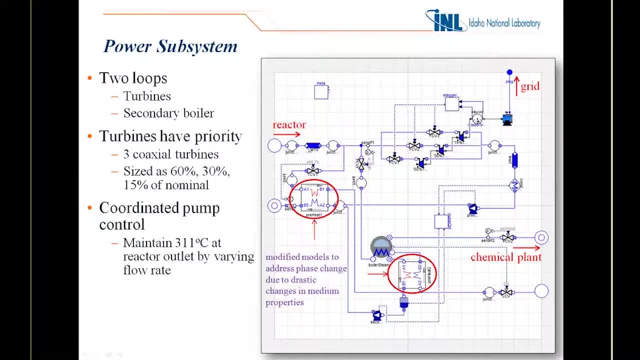 And if you go here, then here you see the different components, the line, the turbines, the generators, Then eventually the condenser here is, as you spin the shaft, here you create a rotational, a mechanical rotation there that is eventually used. 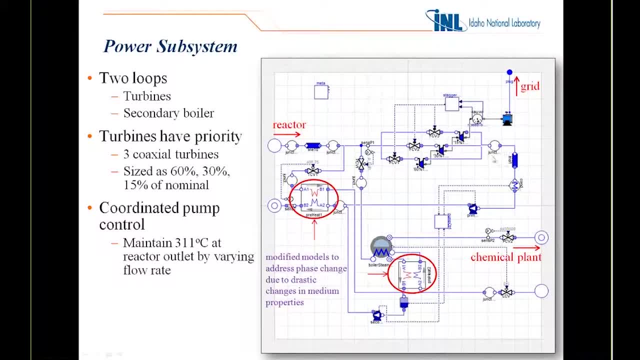 to generate electricity there, Then here, then you have the condenser coming back and going back to the reactor, But then, as I say, some of the excess energy, depending on what is happening here, can be sent to the chemical plant and all this equipment that are needed- boiler reheaters. 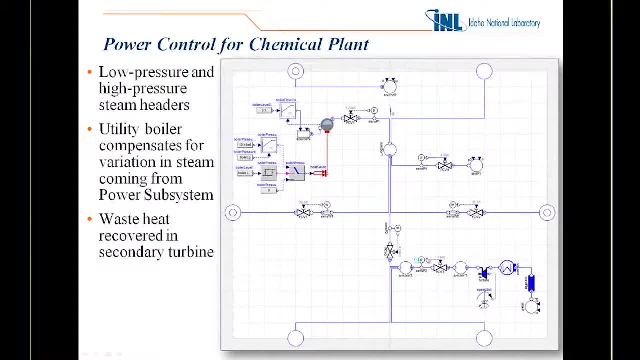 and so forth. Here is all the different models that were put together and developed just to do essentially. you know a lot. Thank you, Thank you, Thank you very much, Thank you very much, Thank you very much. And you can see the headers. 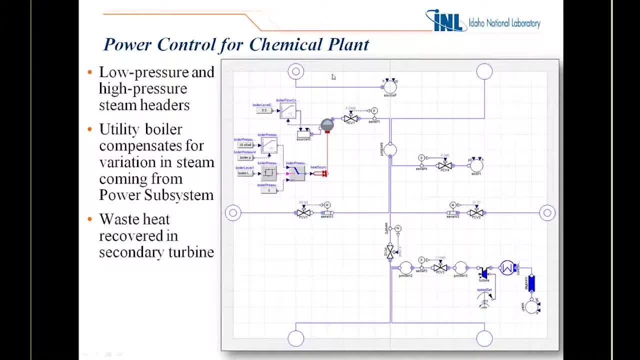 And what this guy does is: eventually, here is the energy coming from the reactor, Here the energy, it is going to the chemical plant, And what all this thing is doing is trying to maintain a constant energy supply to the chemical plants. So we run the chemical plant in some sort. 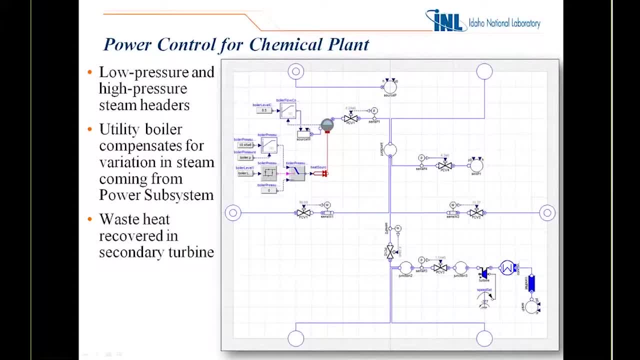 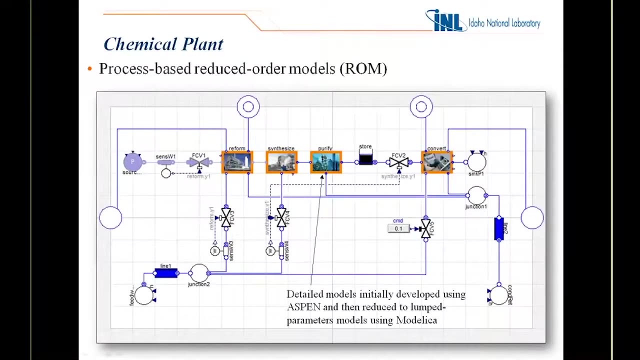 of steady state kind of thing. This portion here is essentially utility boiler that are allowed to compensate for changes on steam coming from the nuclear reactor, the energy, the reactors that be sent to electrical generation. and here is then now the chemical portion of the system, in which you have a different component. 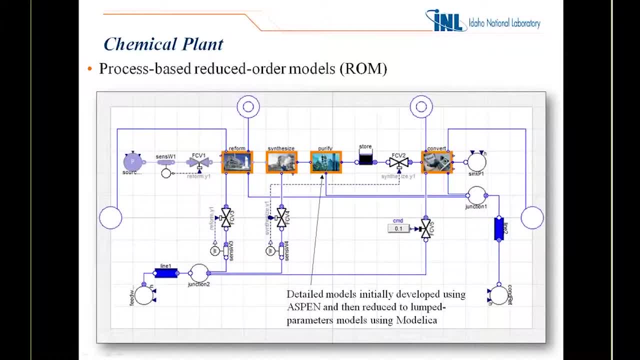 again for this particular analysis. we were taking natural gas and converting that into gasoline here, and then you have a different main element: reforms in the team: beauty. one of the key portion that we did here was, again: all this one was bottled in detail using Aspen and eventually taking those. 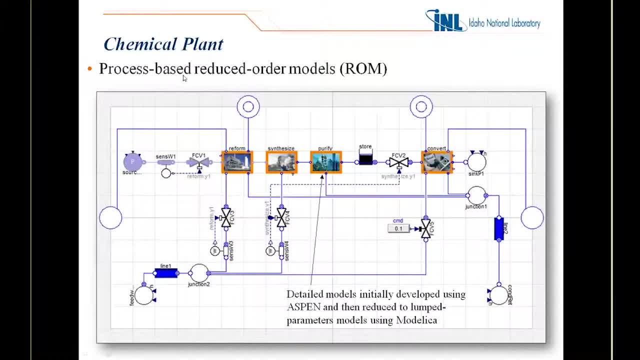 models with computer use, our models, to be able to include in in this particular one. one more thing in notice also is the Aspen model with steady-state, and then we add the dynamics to them and when we integrate in here. I have a question about that. can you give some insight in? 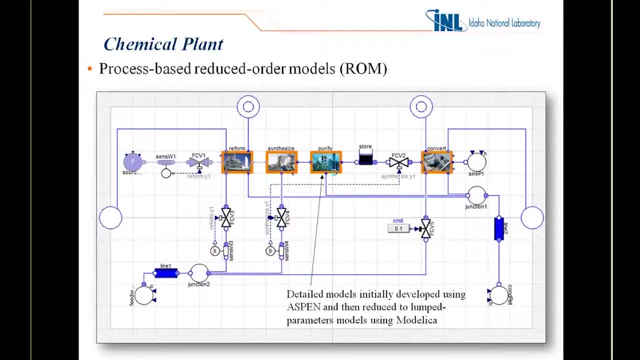 the. Hi, I'm Chris from Alton. I'm from Alton and I was just wondering what are the the deviations you saw between the reduced order model and the detailed model? I couldn't hear well, or we could you say that again. what are the differences you observed between the reduced order model and the detailed model? 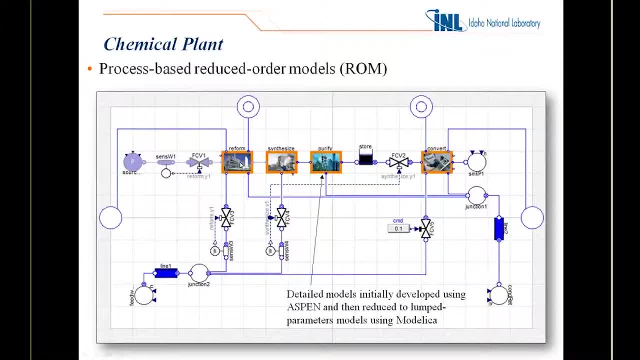 yeah, well, this one, each of these one, very- it was very, very, very complex- and put those models there in the mean simulation. they would have a very long time to be able to converge to anything. So what we did was we took these very detailed models. 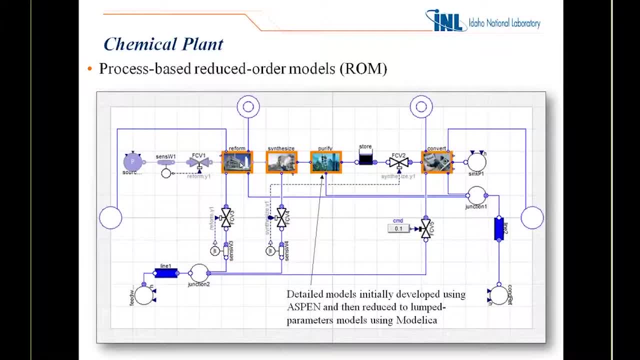 of each of these elements and excited them, saying OK, how it would change with this kind of signal, How it would change. So eventually, given those ones, we were able to simplify that on a first order, differential equation, essentially defining what 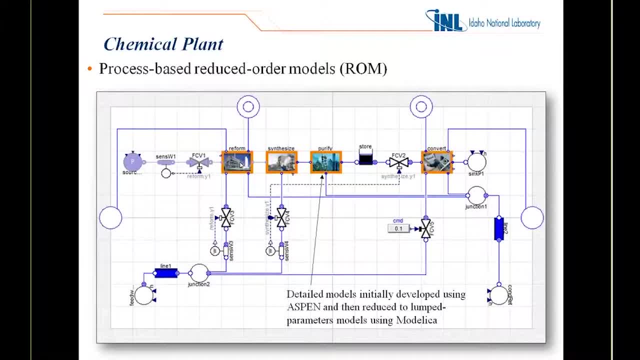 it is the gain on this process. and then, what is the time constant of this process? Same for this and same for that. Now we are working in a more analytical way on resolving this problem, And this is an ongoing effort, But essentially, that's the way how these reduce. 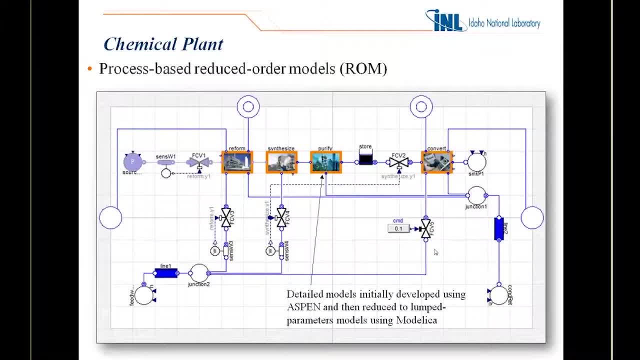 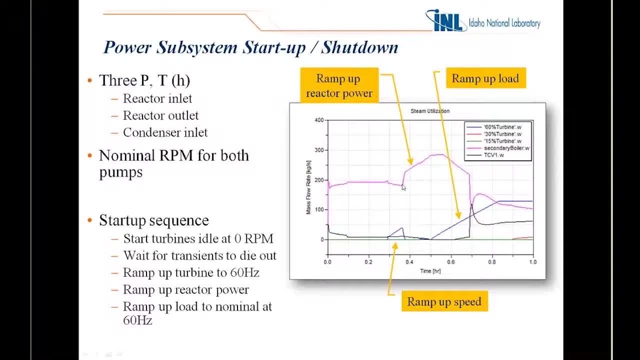 all the models, OK. so here is because of the time I wanted to keep going, And the intent of this is a lot of work- to show the very now complex system one is creating. It provides a lot of benefit to it. 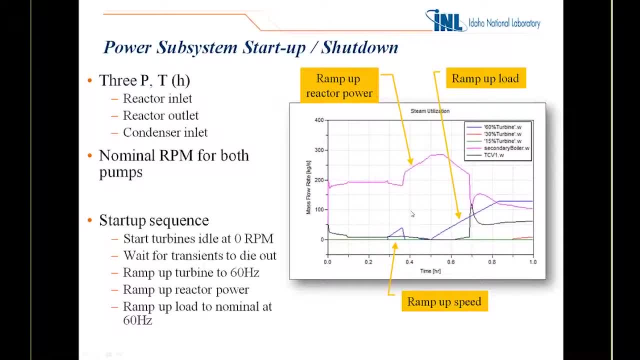 But it requires also to do the analysis of the dynamic, how the system is ramped up and how one's wall will shut down. The intent of this is to show that a dynamic model is needed to be able to understand if I'm losing a sink, a heat sink. 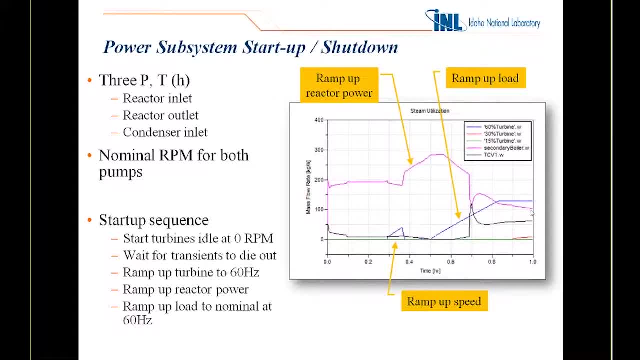 or I. actually a new rule or renewal will come in. One needs to analyze that problem in dynamic setting to be able to see whether the seating is able to react to those changes And if it's not, what kind of mitigation can be put there to accommodate that. 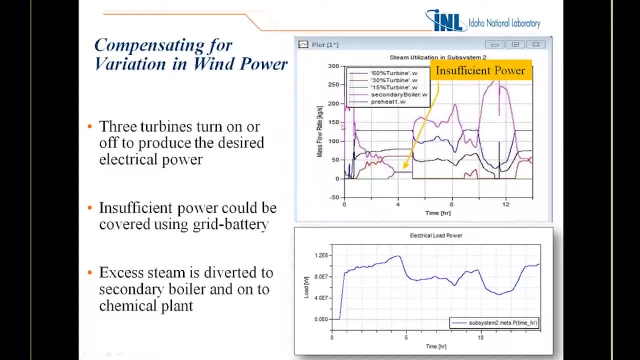 Here, for example. here we see how, for example, here, the different turbine, if you want notice, there were a set of three turbines of different size And here it shows you how the different turbines, the flow going to those two, are in changes. 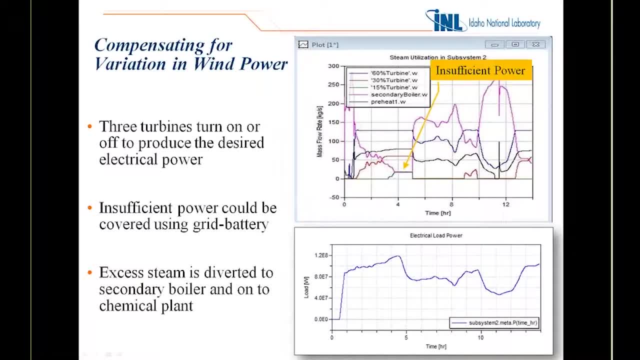 depending on how the wind is changing in a given period there. So you see there is a lot of issues there. This is another example here that I can go later on if there is a time is here. it shows that, for example, if the particular model that we put there 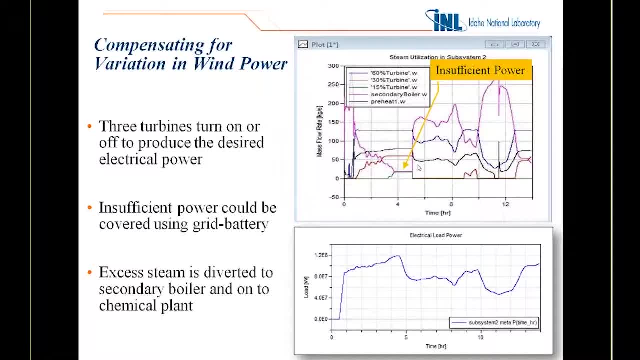 didn't have precise a battery there. So it shows that in this period of time, with this form of wind profile here, we will have no enough power for the system to maintain operation there. So then things like this is that you can only see it really when you do a dynamic model. 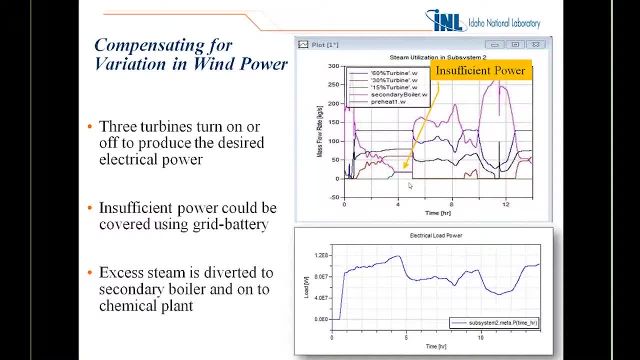 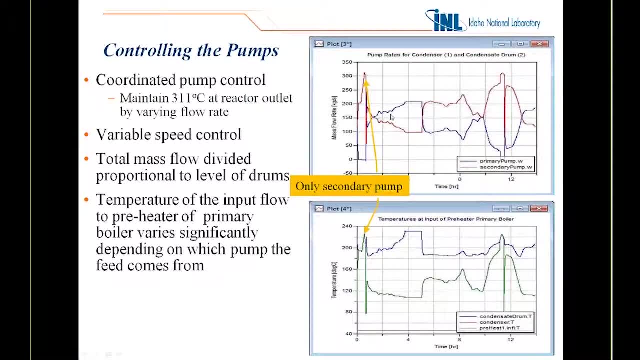 simulation of the particular system. Then here is the controlling the pump. Essentially, here, you see, is the reason that you have here, you have the primary pump going up and down, And this one, almost the reverse of the other one, is because, again, you have one loop descending. 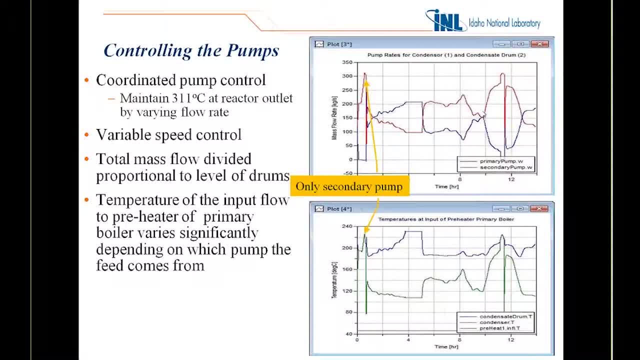 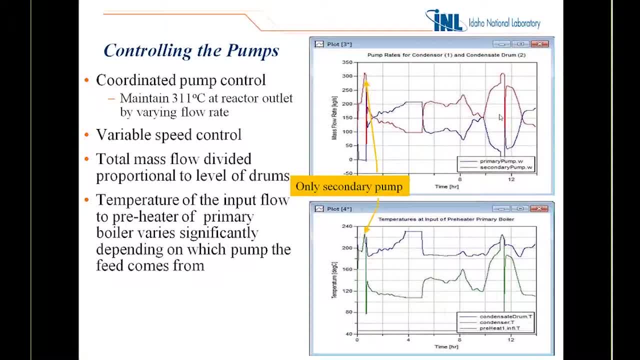 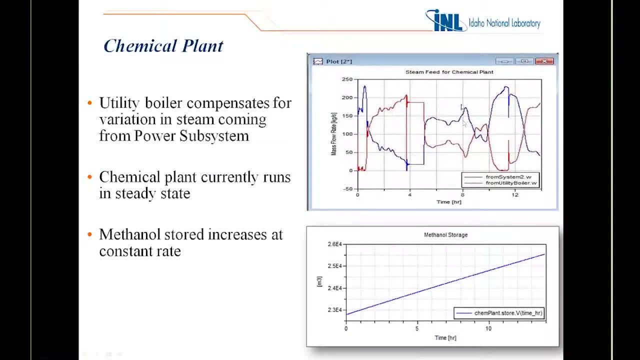 Because, with the assumption here, the reactor is running at the same power level. Finally, here's what is happening in the chemical one. It's the same thing: steam coming from the reactor, Steam coming from the reactor, and it's compensated for the steam from the utility. 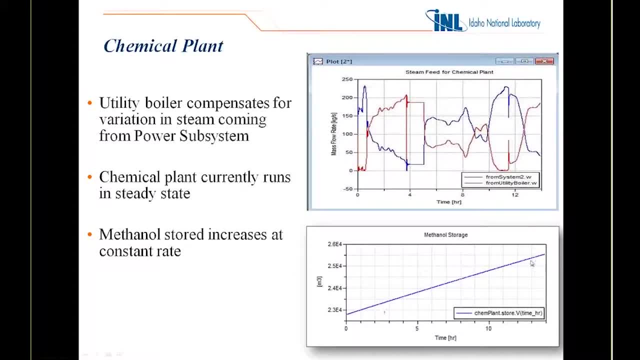 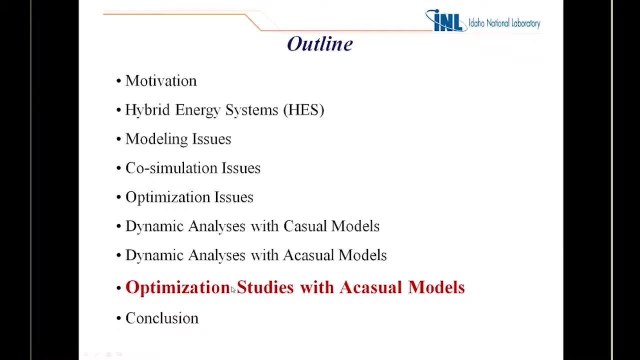 And, at the end, what we want is a constant operation chemical plant. Finally, let me go Dana on the optimization study. So again, so you analyze the system, it works, and now you want to optimize the design, both in what are the particular configurations that you have, the size. 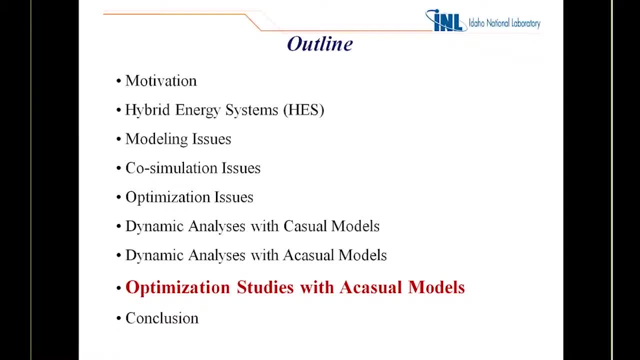 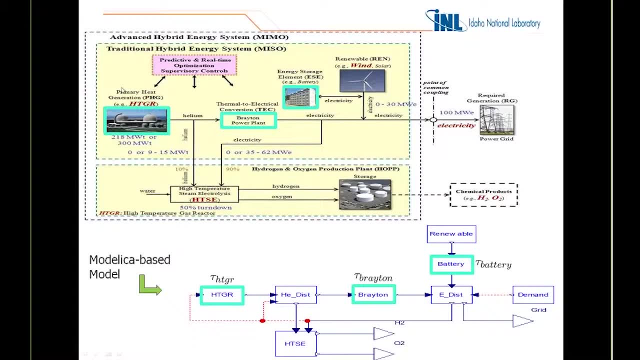 of the elements, things like that, and eventually, how to operate it. Okay, so, Dana, in this particular case, we took this one. This is another Havarin system and you see, a nuclear reactor. It was helium and, John, this is the one you were asking. 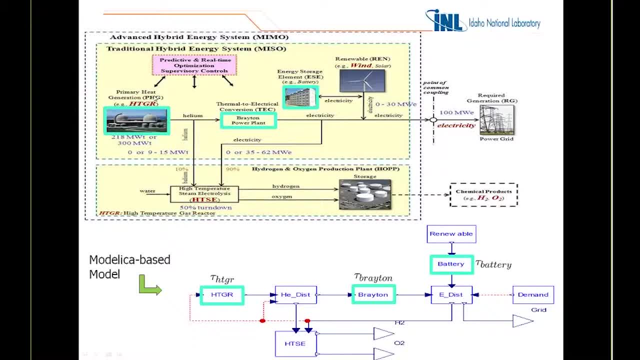 before and let me just go into that. Essentially, you have a high temperature gas reactor, produce helium. it goes to a very important plant- electricity- and then to the grid. And now it is complicated by adding a renewable source, in this case. 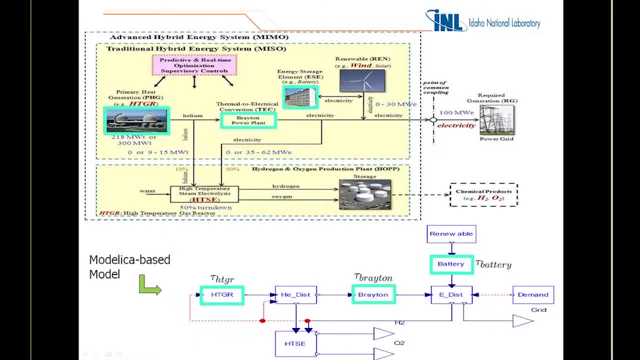 wind, and then we know there's some element of storage is needed. We want to in many ways actually even minimize that. Okay, but Dana will recognize that if there is a lot of variability here, a lot of variability here, then well, you might. 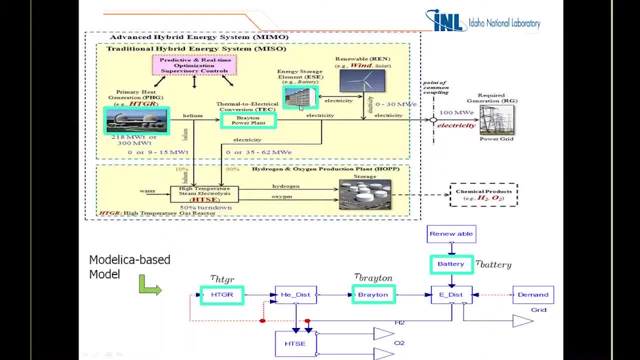 have a lot of variability here and then, well, you might have a lot of variability here, and then, well, you might have a lot of variability here, and then, well, you might have. you might need a big storage air Or be able to modulate the. 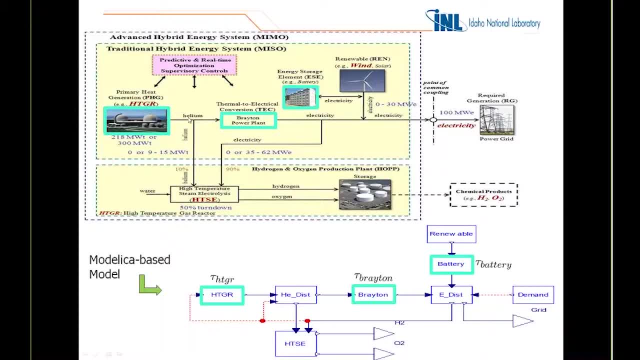 electricity distribution and modulate the helium distribution and utilizing the success coming from this one around the high-temperature stream electrolysis right there. So that's what you saw, John, on the block diagram. The nuclear reactor is generating helium that is being used for power generation. 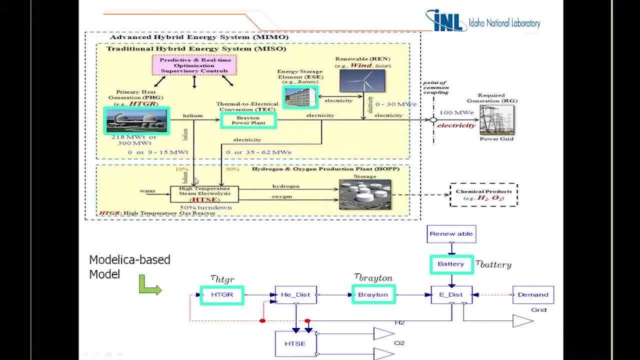 but also helium that is being used for chemical production, in this case, hydrogen and oxygen, right, okay, yeah, that makes a lot more sense. before I'd seen electricity coming in and helium coming out, but I hadn't noticed the additional heat that was coming in from the bottom of that block, so that makes a lot more. 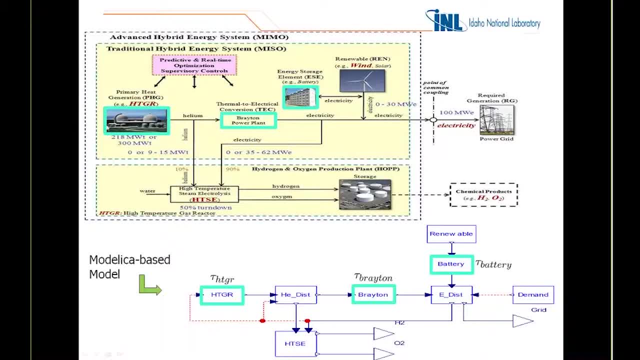 sense, now that you have a full block diagram, by the way, and that the electricity coming here- you saw here- is actually information that you see here. you see there that electricity coming in, it's really a set point telling the high-temperature reactor really how much electricity is needed or really how. 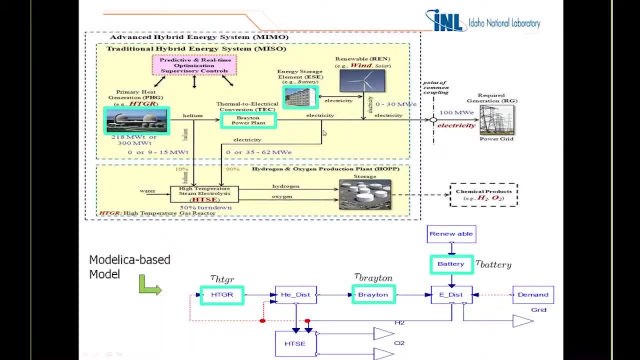 much helium is needed because of what is changing in here and what it might be changing here too. so that's you see here. see, this is the information flow coming here. and then the reactor: hey, here is my demand: electricity. oh, this is my demand in helium for you. and then the reactor. I can only react to that and generate the. 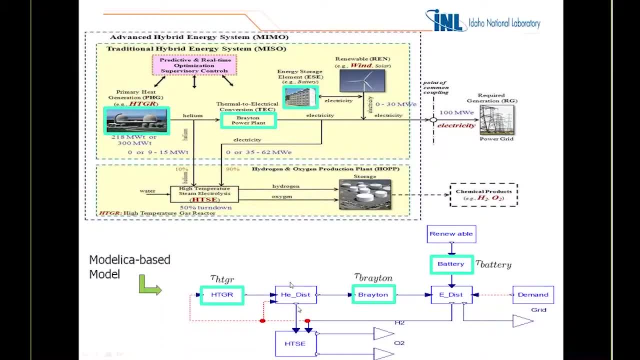 helium. then eventually, you see here- by the way, sorry, here is the block, here is the model written in in the molar and modalica. so here's the high-temperature reactor, here is the helium distribution and it's being modulated. then, if the helium is used, 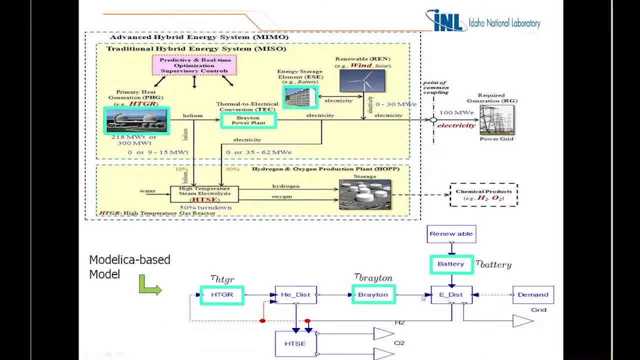 either for power generation, but I remember, here you are electrons, electrons here, but this is modulated at the same point. that either goes to the grid or it goes to feed the high-temperature chain electrolysis. and there you are. so this is the model on modalica. now, one interesting part of here, by the way, here's some particular but one interesting part of here, by the way. here's some particular but one. 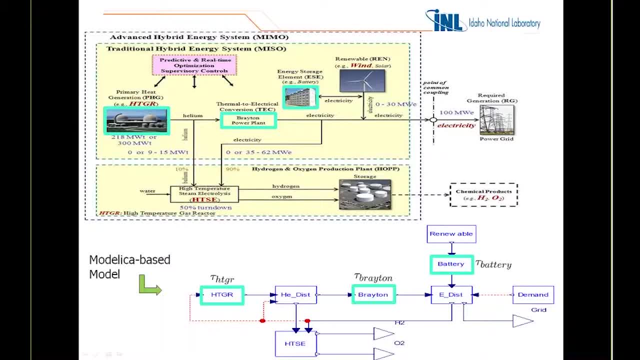 of the key theories that I have used this. okay, there is no more to do about this one of the keys. the reason I'lls this is because in essential, it is a chemical plan that can nicely fast react to changes, because most of his inertia come from electricity. there it's not really. 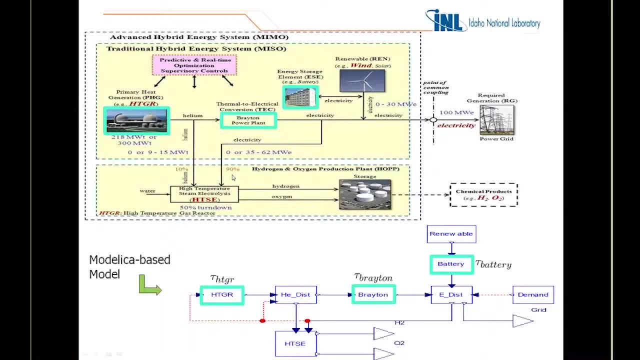 thermal. look at the ratio between electricity and a thermal thing. so because it's mostly driven by electricity, this guy can react quite nicely and fast, given there were energy supply chances anyway. so the question that we're having here is okay. now let's assume that a marry if we thought em is actually a taste changing here. 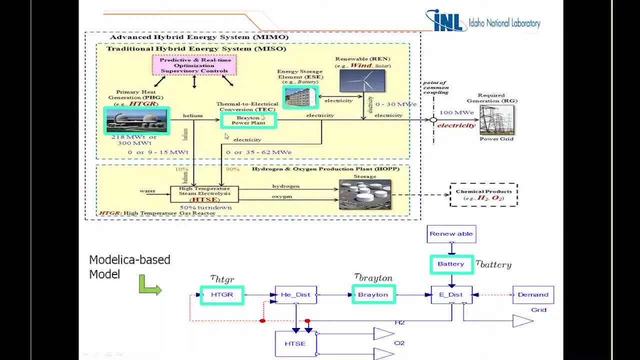 We want to design the reactor here and design this one, and design this one, and we want to see how fast the dynamic needs to be to accomplish certain requirement on the certain constraint. Well then, what we did? we put this configuration. 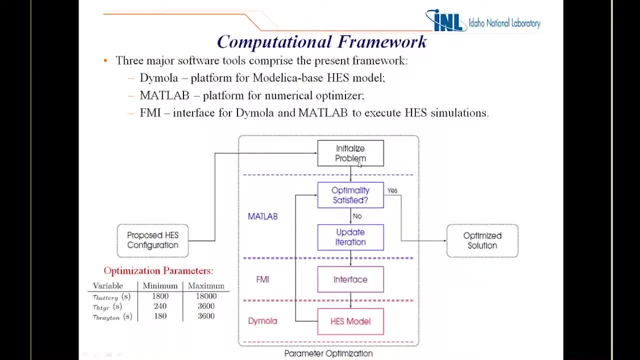 this framework in which, so essentially, it was an optimization problem, right? So in doing that is okay, given that somebody provide an hybrid energy system model or configurations, what are the values of these time constants that are needed there? So the problem comes in here. you say: 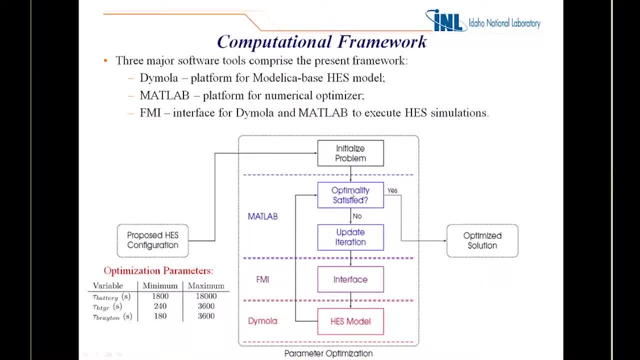 okay. is the particular set of value a medium optimality that we want to certify? If it's no, then we upgrade iterations, then we send that to the model, run the model, see how the model responds and then we check some metrics. 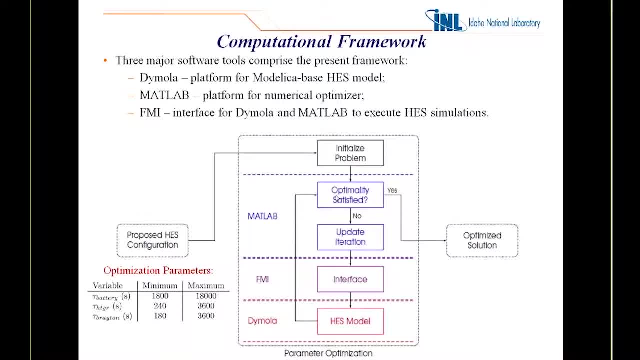 We achieve the cost function, we minimize and we optimize the loss function we're trying to optimize. If they ask me, I'm like: okay, this is we're done. If not, we can't do it. I think one of the important part here is also: 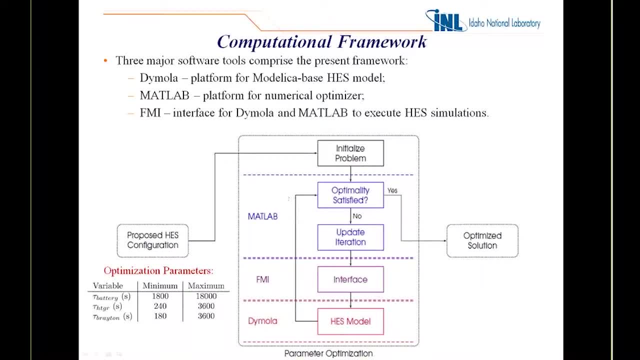 to show the different tools that are required here. Tools, for example. here is where your models actually live. In this case, it's a model Modelica. Here is where your optimization algorithm live. In this case, we were using MATLAB. 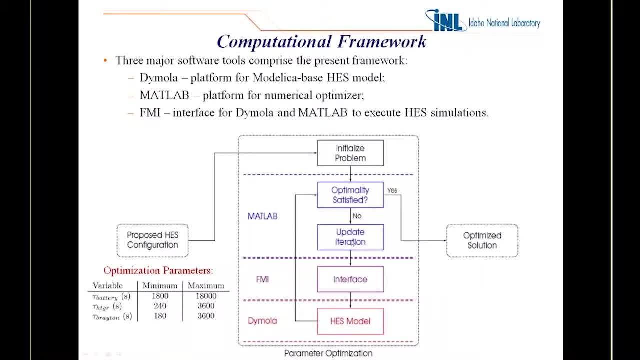 and a series of algorithm we have developed in collaboration with our university. And then you need something to connect these two worlds, the world of MATLAB, to the world the model, and this way we use the FMI, Which is getting more and more and more relevant in here. 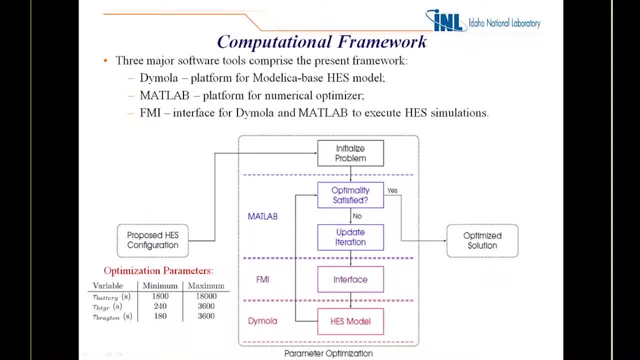 Again, remember that what this block does is trying to figure out what are the optimal value for the time constant for the battery, the high temperature gas reactor and the Brayton cycle, And we're given a minimum maximum defined by the particular technology limitation. 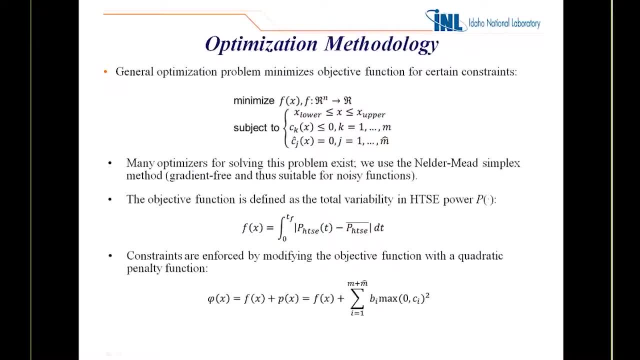 that the system can provide. Okay, so here's the loss function we're trying to. well, actually, this is the optimization problem that we're trying to achieve, It's minimize this loss function, Solve it. so a combination of both equality or inequality, constraint there, as you see there. 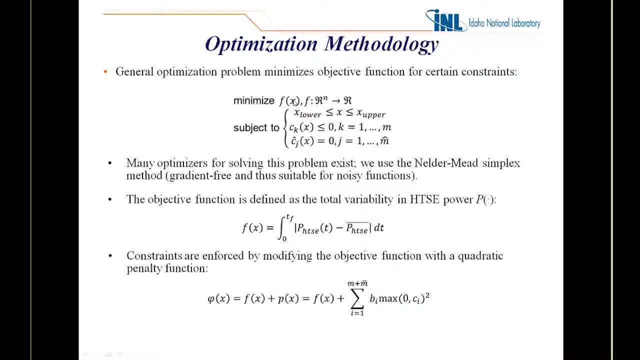 Right, and in the particular one here, the loss function is given by this equation And this one essentially says: hey, we want to minimize, we just want to minimize the viability of electricity. going to the high temperature stream, electrolysis, Because even though this particular chemical system 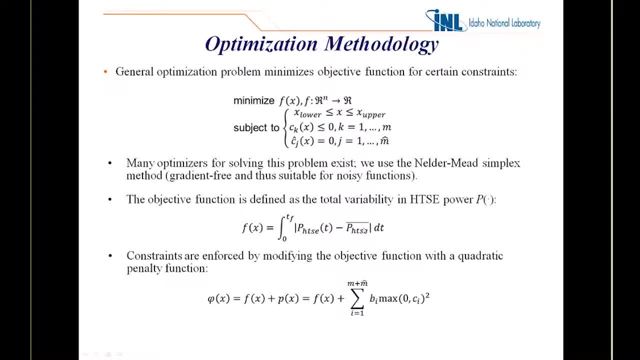 can react nicely to changes. we want to minimize just that. Okay, now we modify that one to inject the in one single equation, the constraint by this artificial in here that you have in here, Okay, so rather than going to this one, 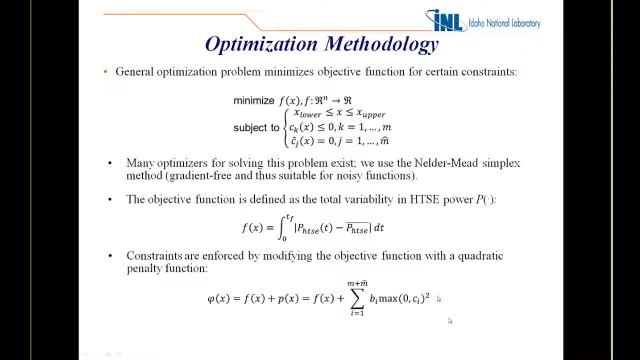 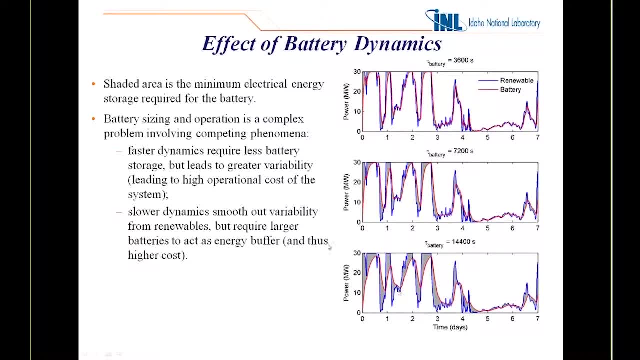 we're going after this one and do the optimization of this one, which have both the initial loss function plus the constraint, Okay. so then, in doing that, we say okay, well, let's see how different values of how. 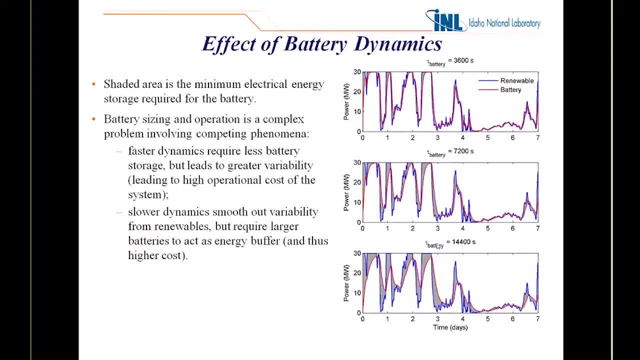 of the effect of the value does in smoothing the signal, going into electrical production And what you see here, for example, that has here you have, for example, here is the value, here is the renewal, And remember the value, what it's trying to do. 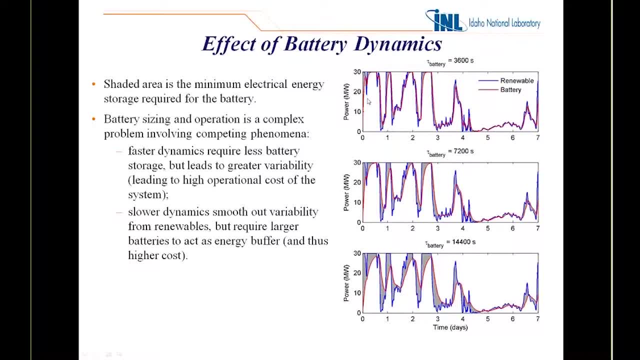 here is the smoother signal. So here you have, and here you have- a very small battery, that is have a very storage, because the shedding area is how much energy it's storaging As you increase the size of the battery. so you require, okay, the signal coming from the renewal. 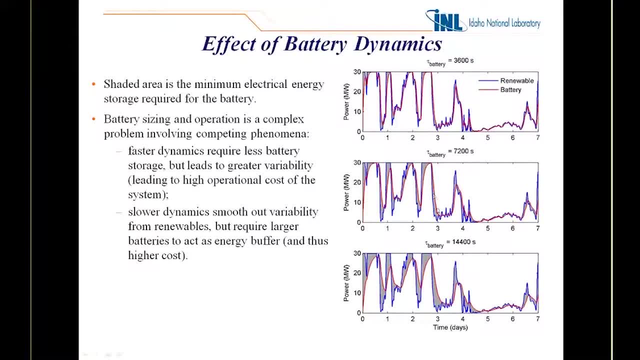 is smooth more, but then the shedding area require- okay, now the type of the battery you have, and then here you have one which is more smooth, signal, but they require all this gray area, the storage by the battery. okay, So increasing the body in this direction. 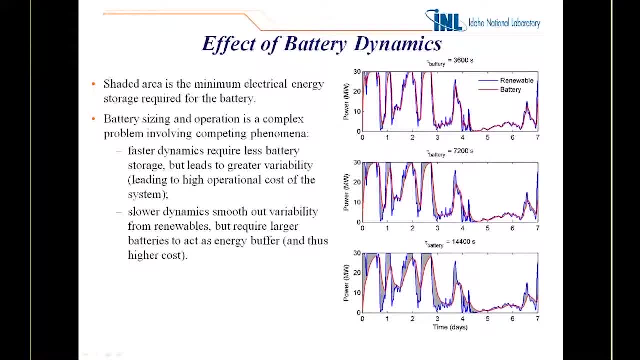 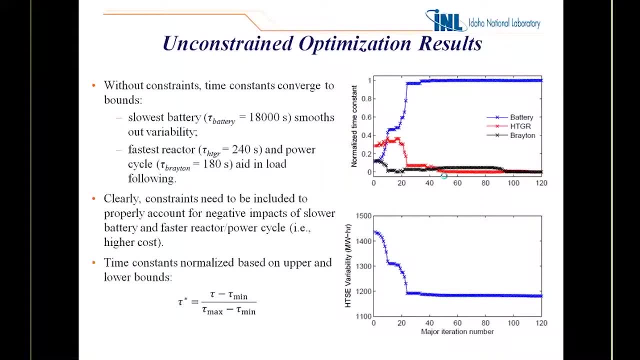 Okay. so then? okay, so recognize, yes, that the body does have a good function there, but then let's see what is the optimal value of this particular dynamic setting. So what we did is okay. well, let's put that in an optimization problem. 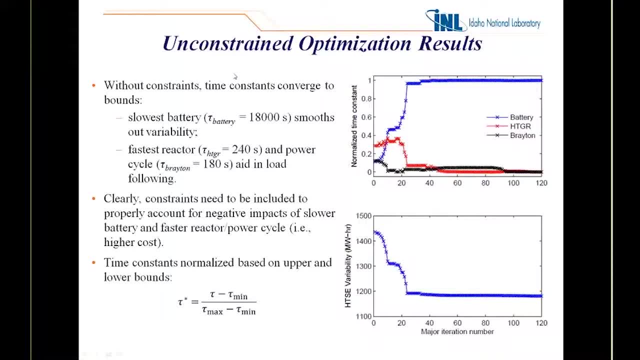 and then let's try to find the optimal values of the system, but then let's do it unconstrained. Well, what this plot shows in here is: here is the, the optimization iterations, and here is the values of each of these: the time constant for the battery. 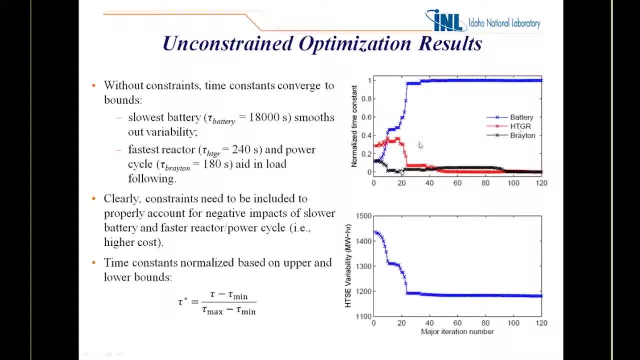 for the high temperature gas reactor and the Brayton And what this one shows. they essentially all go to the limit. The battery goes, tends to go to the biggest battery it can go and the Brayton and the reactor to the fastest dynamic they can go. 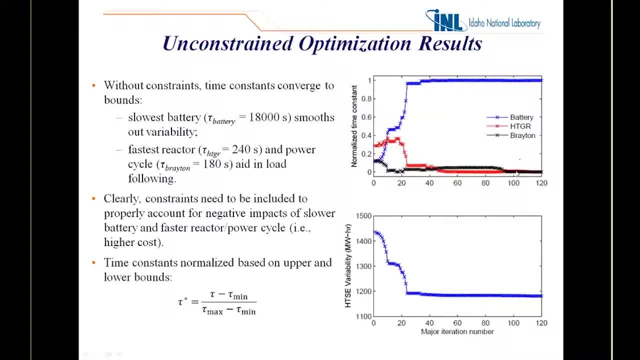 So I mean it's an obvious result. Is that optimal? Possibly not, and that's why you will see later on the constraint, By the way, here is here. like I say, here is how you go in optimization. 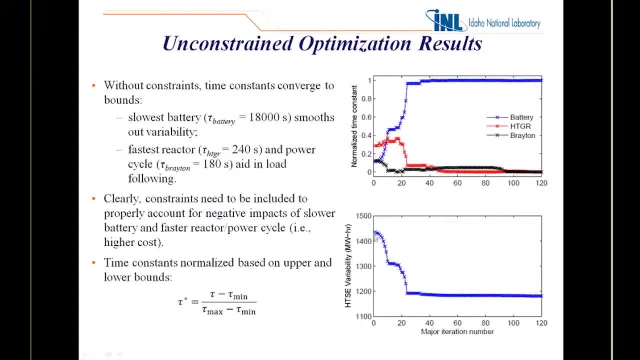 and here is how you is the low function I just showed you, shown from a maximum value and eventually goes, and this is the best value you can get in availability on the electricity going to the high temperature electrolysis. okay, So the unconstrained is not exciting. 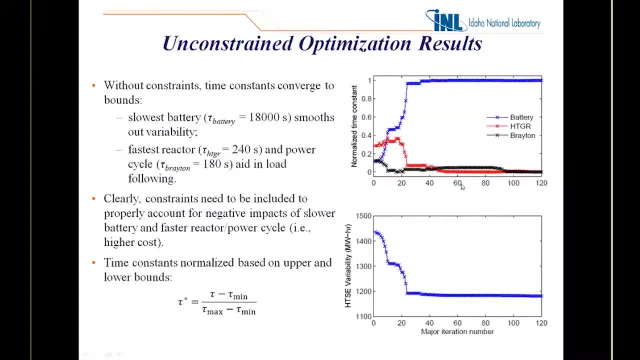 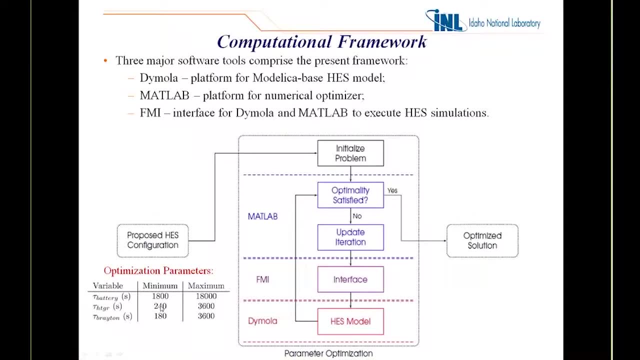 because it gets us to what we thought was obvious, which is again goes to the maximum into the battery and goes to the minimum into the high temperature gas reactor and the Brayton. Obviously it goes by itself. They say: well, it's a way, a better, optimal value. 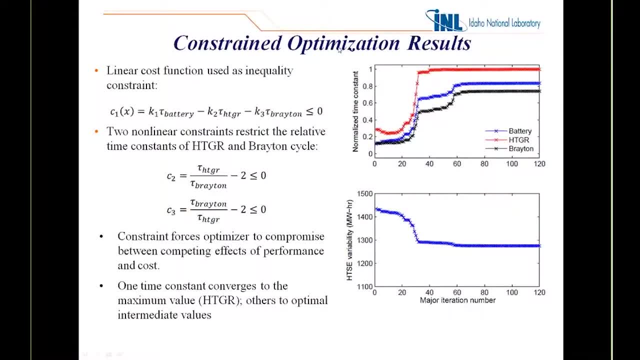 so then now we have the constrained optimization result and then now we put a discussed function here in which now we weight the different these depending on the technology. In this particular one we were saying, hey, we put K2, actually four times more than this. 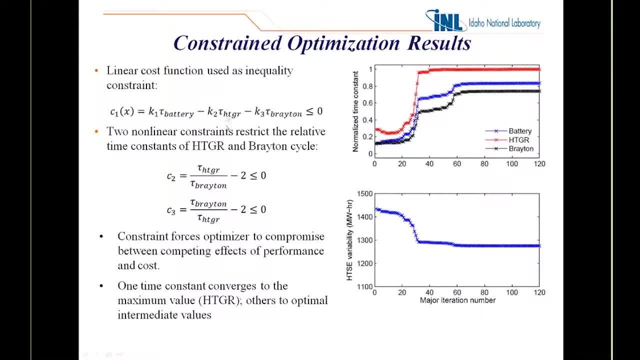 and this one to show we don't want the most variability in the high temperature gas reactor. Try to see whether that variability can be passed into the battery and the Brayton cycle. And here is, essentially, bounding from the top and from the bottom, the difference between 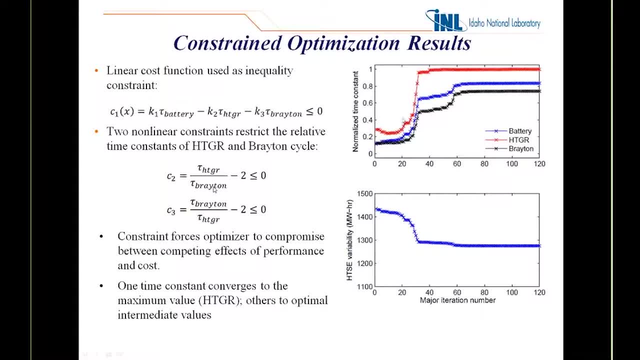 the high temperature gas reactor and the Brayton cycle. Okay, so now the result is quite different now. So here is the optimization path, and then here the values for the battery, the high temperature gas reactor and the Brayton cycle. 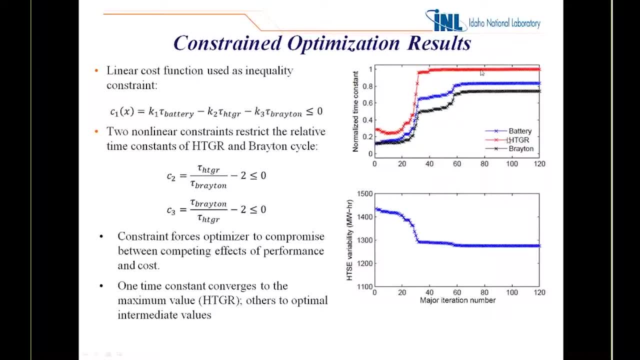 And what it shows there. yes, the high temperature gas reactor goes to its maximum value, but now for the battery and the Brayton cycle. now it doesn't go here where it was before, but now some intermediate values there, And so that meets these constraints. 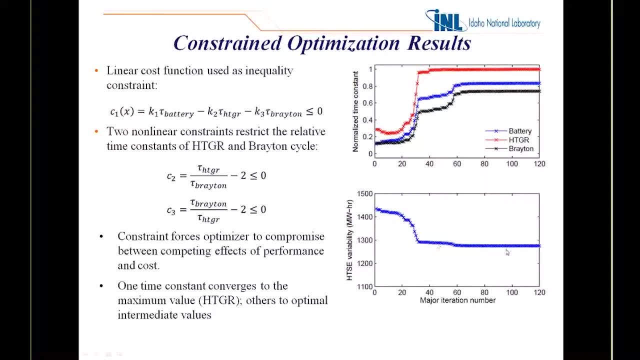 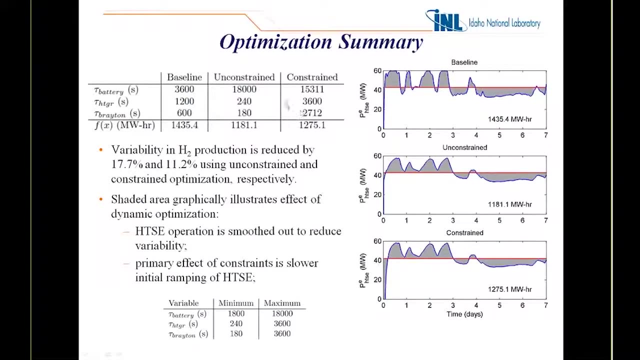 and then, as you see, now, here is the variability of high temperature gas reactor, of the high temperature stream electrolysis. We optimize values of the for each of these elements, And okay, so then here is the. again, the constraint went to. you see the summary. 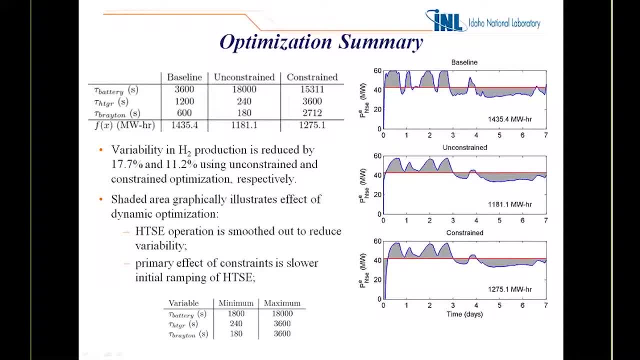 The constraint went to the maximum here, but now the constraint goes to a lower value, to the lower one, and these ones before were going to the minimum values, and now they get a value in between those two. Okay, and here is the response of the high temperature. 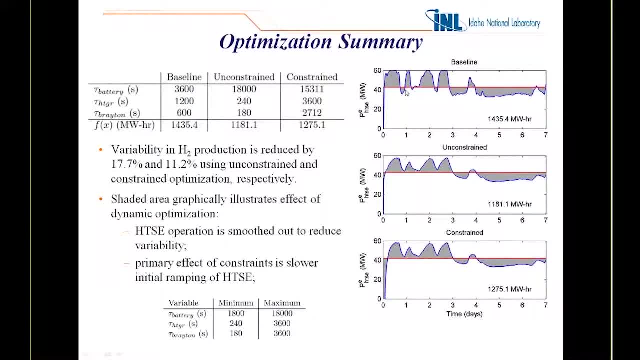 stream, electrolysis, The wave of the power going to the device. So you see how it changes on the constraint. Essentially, what it changes is how the CT initial react when the whole process is put together and when the wind comes in, and so forth. 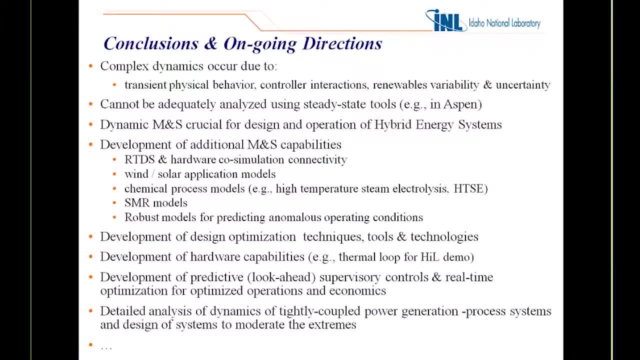 Okay, so finally to end this presentation, Dana, so the I think it's all you see there. there is a complex dynamic because there is a trenchant behavior on all these different components, how the controller interacts, and then also the variability introduced by renewable. 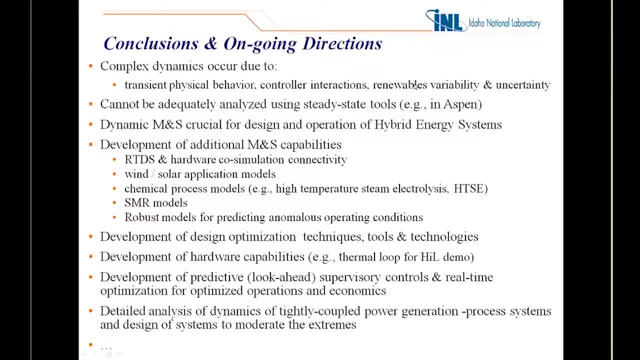 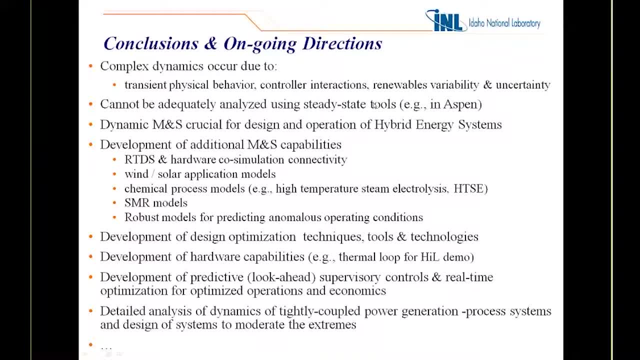 that they cannot be analyzed using steady-state tools. just Aspen Tool can be a way to actually this kind of tool is a way to reduce the number of candidates, but eventually we need a dynamic analysis of the system. So the as an indication here. 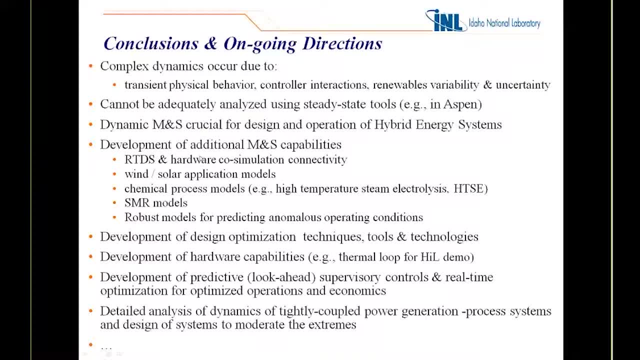 so, and then what we're doing now? so, then, co-simulation is an important one, and, recognizing that we have unique physical assets here, then we're creating tools and be able to co-simulation between software and a specialized system like the RTDS. 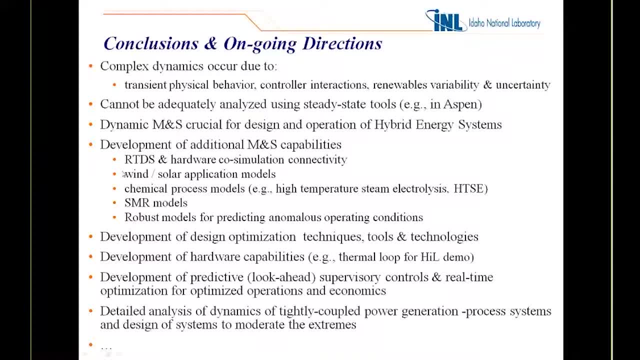 Then we are, for them, making more detailed implementations of development of models of renewable, and these will be models, a course of models of wind and renewable wind and solar. I think in here we need a lot of help here, A lot of the models that we have. 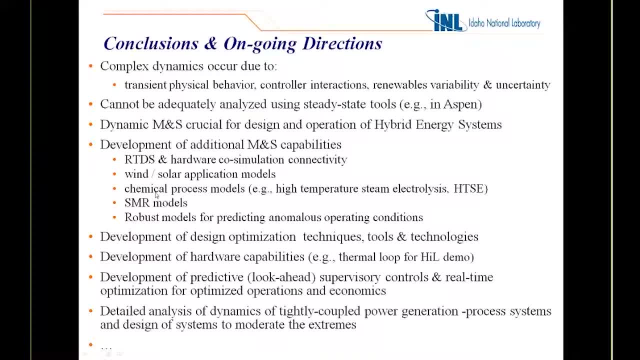 chemical process models are steady-state, Many of those one, Aspen and so forth. Be able to have dynamic models of chemical processing is key and an important one, and even more, it will be even nice to have a course of models. 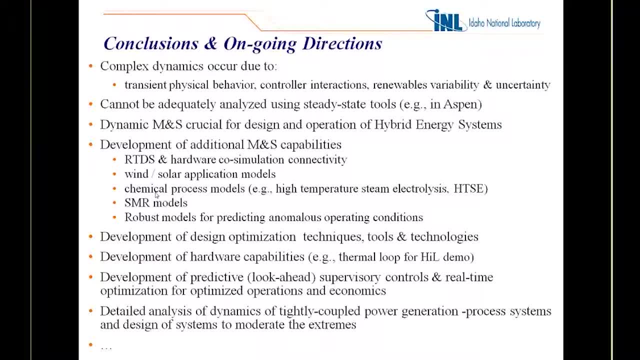 dynamic course of models of chemical processes. We have been developing models of small-model reactors and then that can be used to predict another model of critical issues and other normal situations. As I was saying there that we're working on optimization techniques, tools and technologies. 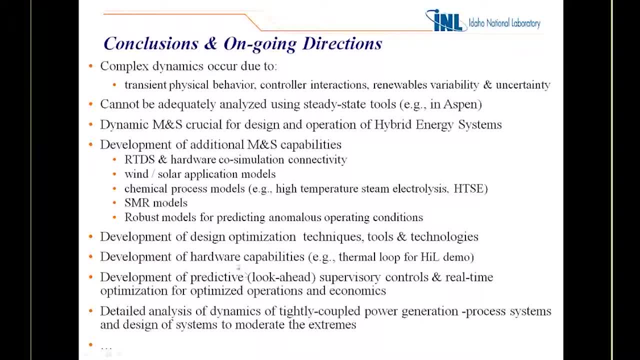 Then developing a hardware capability which will be able to do this hardware-in-the-loop simulation. that will provide more realistic analysis for what we're doing. Then again, monitoring and control is key, and be able to do predictive control is an important one. 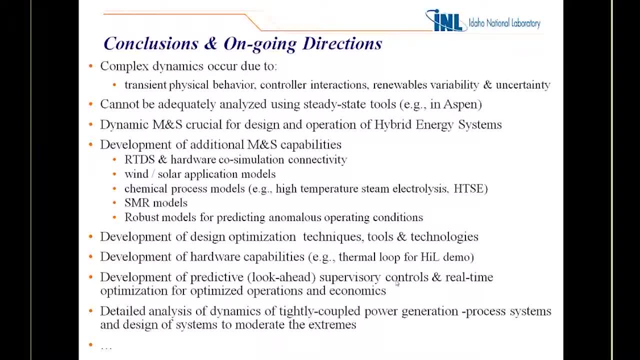 especially in one input, in the renewable generations. And then I do more detailed analysis on this kind quite complex systems to be able to understand them better and to identify what are the technology gaps that ones need to be addressing, Like, for example, do we need a different type? 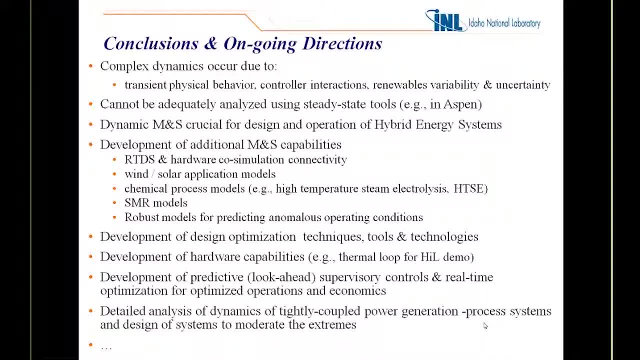 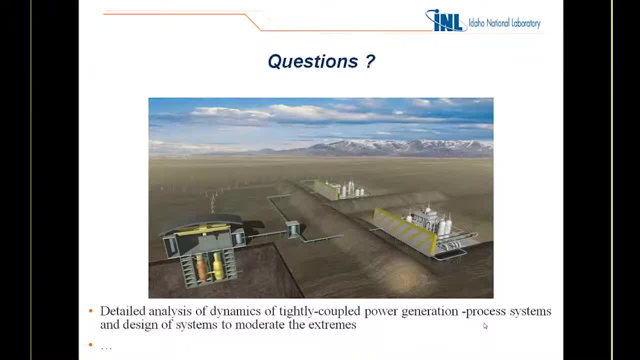 of heat exchanger that allow more easy, more utilization or changes of thermal energy being generated. But with this, that ends my presentation.